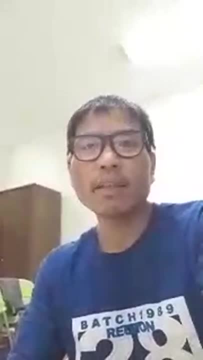 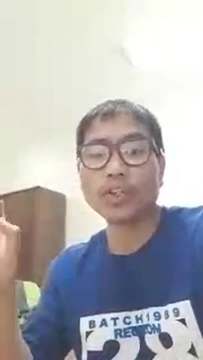 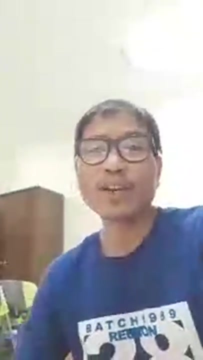 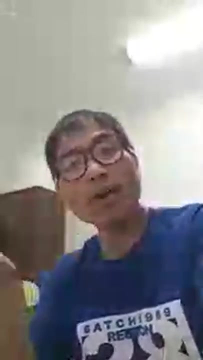 This may be helpful also, okay, but not so much in that The more important is to learn also the you know the radiography process, The radioactivity, right, the radiation processes okay. the alpha ray, the alpha emission, okay. the alpha decay or any radioactive decay of nucleic atom, okay. 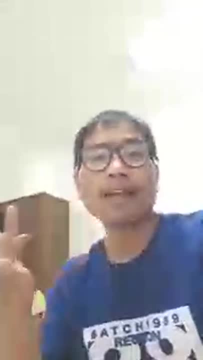 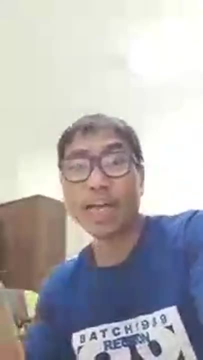 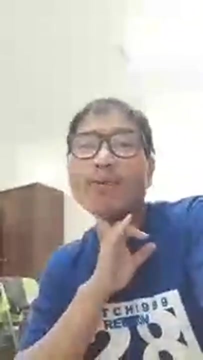 If you remember those three right- the alpha, the beta and the gamma- okay, you have also to take note of that one. And then also a little bit of half-life reaction also needed here. But don't you worry, we will not be able to go to the most complex discussion, okay. 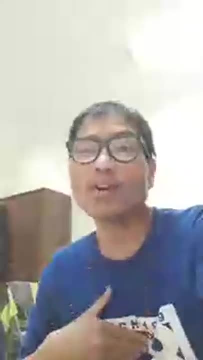 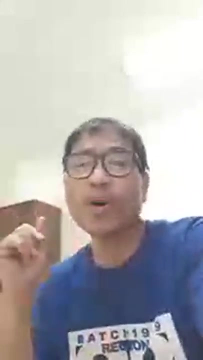 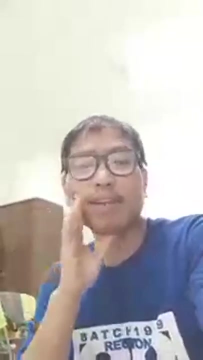 So me honestly, really, this is one of the difficult subjects in Bachelor of Science, in Chemical Engineering. okay, I don't think so if this subject is also a part of BS Chemistry, but I doubt they have also this subject, okay. 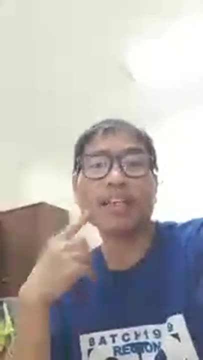 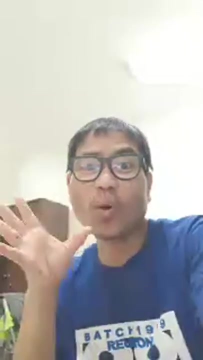 Any BS chemistry students? There you have this subject: Chemical Reaction Kinetics or Chemical Reaction Engineering. Of course it's not engineering anymore, because they are not an engineering course. right, This is, they are taking BS Chemistry. okay, like that. 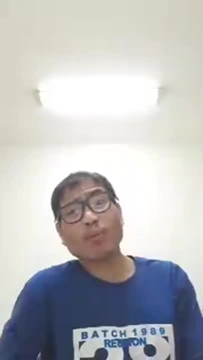 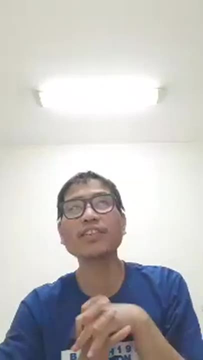 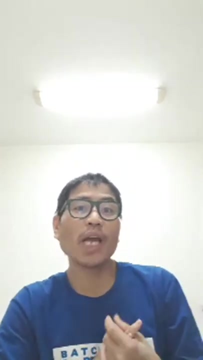 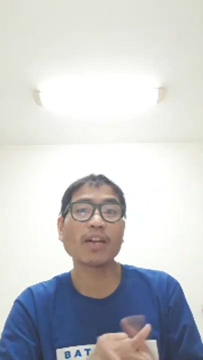 So we don't have to touch particular reactions at this point in time. This is on the overview. okay, like that. and we need to understand the basic foundations of rate low of chemical reaction. rate low of reaction actually rate low of reaction is just equal to rate low of chemical reaction. 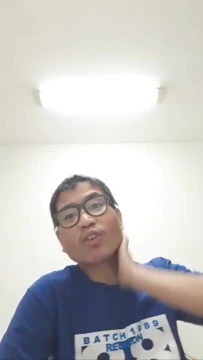 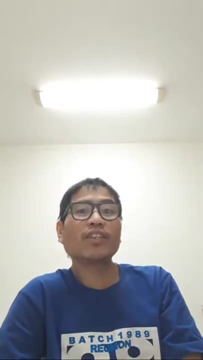 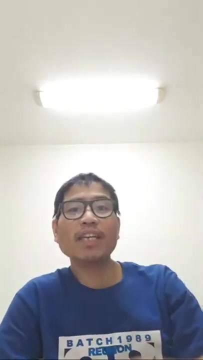 or is just equal to rate of reaction. there are a lot of terms for that. The important word to remember is the rate R-A-T-E, and you take note that if it is a rate, it should be with time in the denominator. 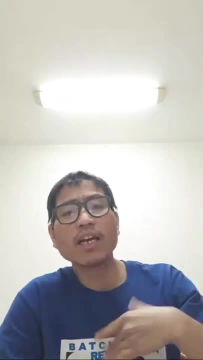 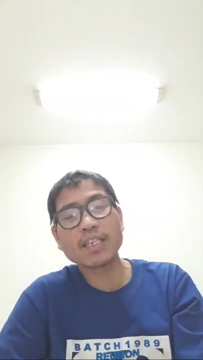 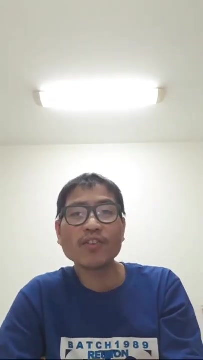 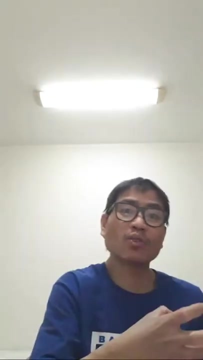 Okay, for example, moles per second, moles per hour, something like that. okay, So this is going to be the rate. Remember that always rate should have always the accounting of the time, the time it takes for the original reaction to proceed, the chemical reaction from reactants to the products. okay, 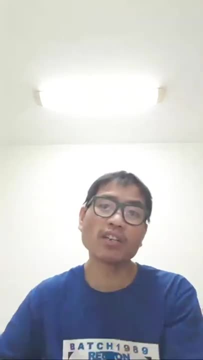 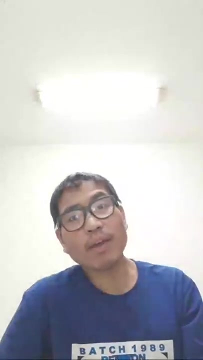 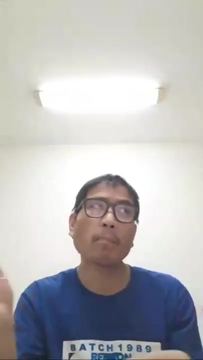 Conversion of the reactants to the products Like that. so this is what we call a rate. okay, And we need also to know about the method of initial rates. okay, Of course, if there is an initial rate, we have also the final rate, but here we are focusing more on the initial rate. 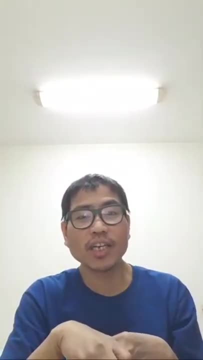 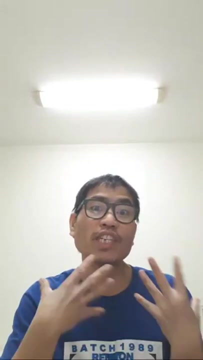 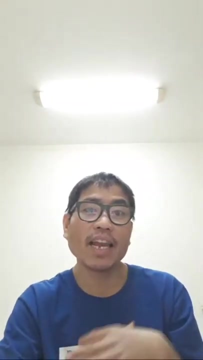 because in this topic, chemical reaction kinetics, we are more focusing on the reactants. okay, like that. And we also know the definition of the overall reaction order. Okay, reaction order in, let's say, element A, element B, or should we say concentration A, concentration B. 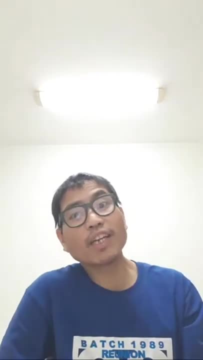 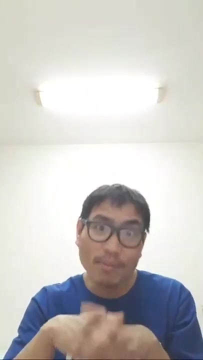 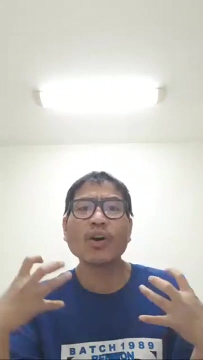 but in here we start to the variable, first or hypothetical examples. We don't deal with exact elements at this point in time. okay, normally gases. okay, in the situations, normally gases. okay. But in here we will be having variables, the X and Y, the B. 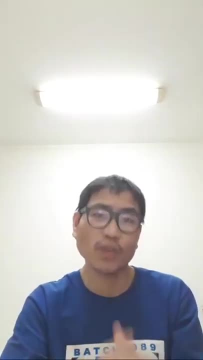 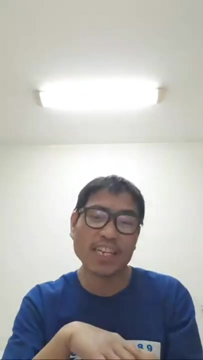 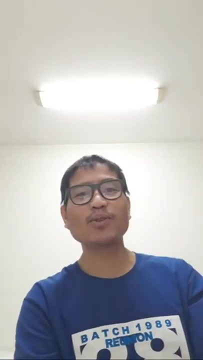 The C, the D variables to consider first, and then we need to introduce so that we can understand further, before going to the most difficult and complex chemical reaction engineering examples. okay, Again, as usual, I will be able to get a blank sheet of paper. 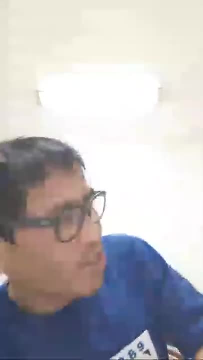 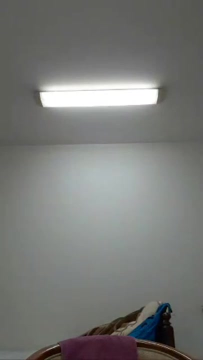 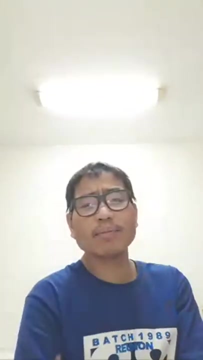 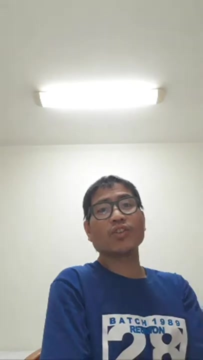 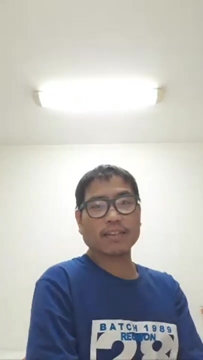 Okay, my timer starts now, oh my gosh. Okay, but before that let's talk about a little bit of half-life reaction, because this is also considered a little bit in studying of chemical reaction engineering. So to tell you honestly, before taking up chemical reaction engineering and chemical reaction kinetics, 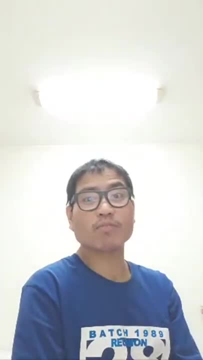 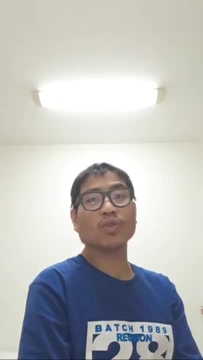 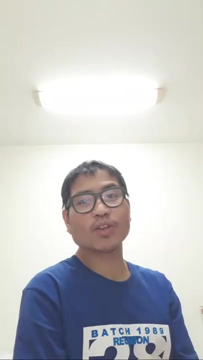 okay, this is the same. that's only the descriptive title of the subject. okay, You have to finish All your general chemistry. okay, one and two, both laboratory and lectures. okay, Before proceeding. this one because these are the prerequisite, because you need to understand different type of chemical reactions. 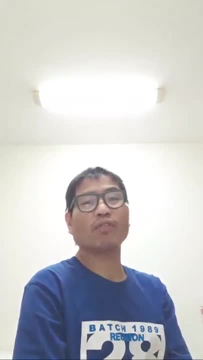 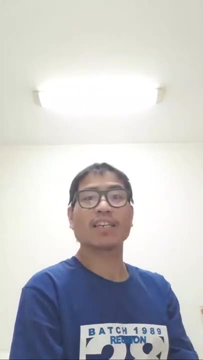 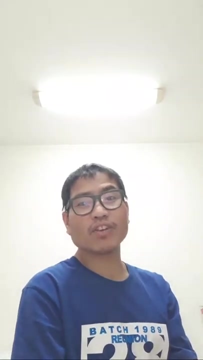 the rate of the chemical reactions, the principles of the law of conservation of energy, the law of conservation of matter, the law of conservation of mass right. So we need to, you know, have Thorough basic foundation and knowledge for the general chemistry. okay, 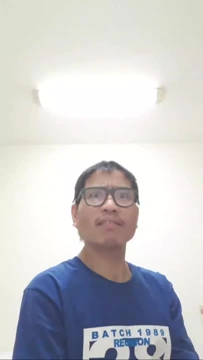 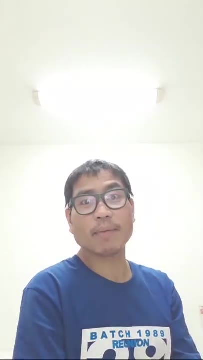 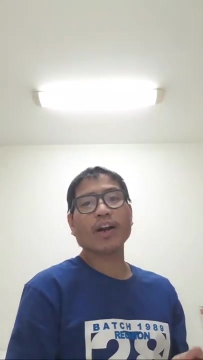 Not so much with organic chemistry, okay. But it's more advantageous if we learn also a little bit of organic chemistry. It could be applied also in chemical reaction engineering or chemical reaction kinetics. okay, So we are now on the chemical reaction engineering. 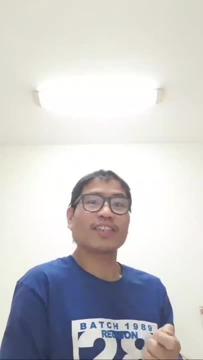 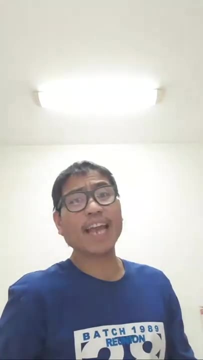 Actually, this is not the chemical reaction engineering. Okay, So we are now on the chemical reaction engineering. Actually, this is not the chemical reaction engineering. This is not my favorite subject, or this is not my favorite subject, by the way. I don't like because, you know, this topic really requires a lot of data, data analysis through experimentation. 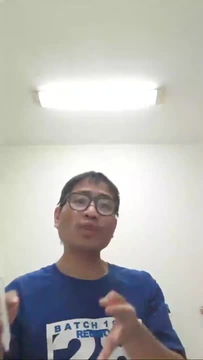 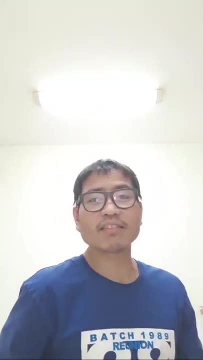 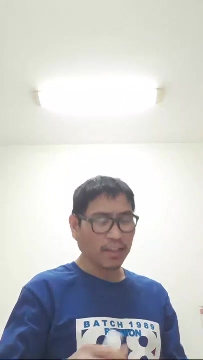 and then data one, data two, data three, data four, and this data will be used in your rate equation, something like that. Okay, Rate low of chemical reaction or rate of reaction, something like that. and you know, sometimes you'll be a little bit. 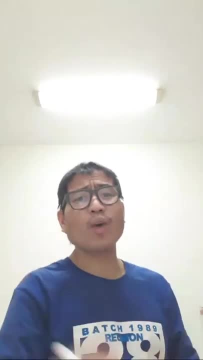 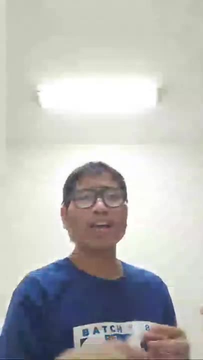 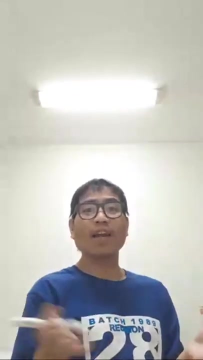 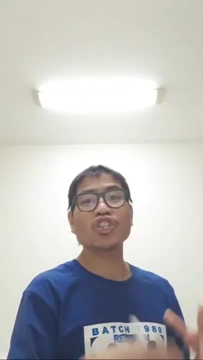 confused if we try to make up with complicated elements, particularly gases. okay, and then you know, sometimes, if you will not have an adequate knowledge of, of course, the balancing of chemical reactions, sometimes you'll be lost. also okay, especially the ice method. you know the initial okay and then the change in. 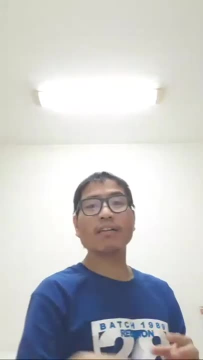 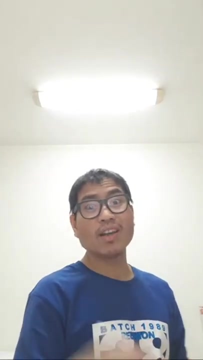 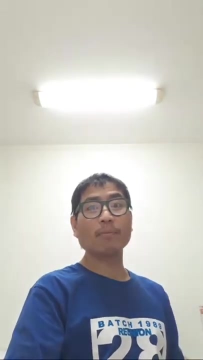 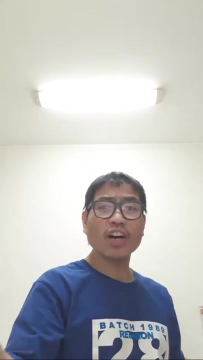 the concentration and an equilibrium- okay, remember that one- an equilibrium constant topic or equilibrium chemical reactions also. and then the idea of equilibrium constant is very important here also. okay, the solubility, product constant, the KSP. okay, the equilibrium constant because the concentrations of the product over the concentrations of the 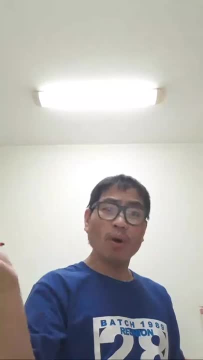 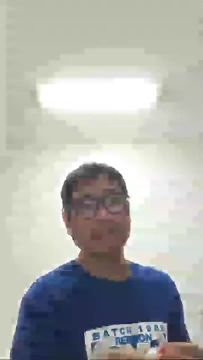 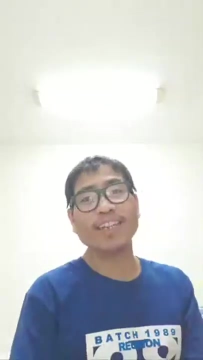 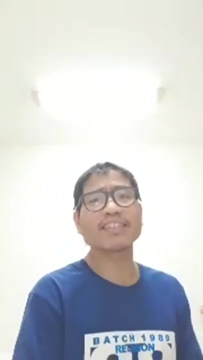 reactant, okay, raised to the number of moles, something like that. it's just because it basically the same here gonna be, you know, a little bit of experimental okay. and then we have to discuss this, clearly, the most basic one even up to now. I cannot really, you know, understand thoroughly this subject. 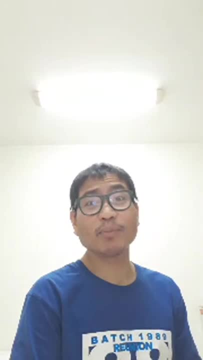 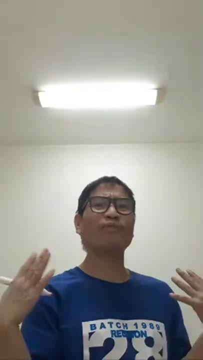 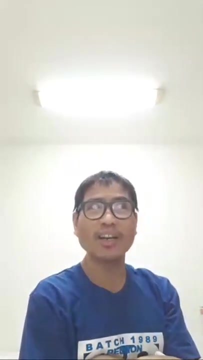 okay, I have only, I think, 60%, but not really that 100%, even though I am already a licensed chemical engineer. but still I have confusion, okay, and so my chemical engineering is my highest score in the board examination, which, chemical reaction engineering, is also a topic there. but you know, this is not really my. 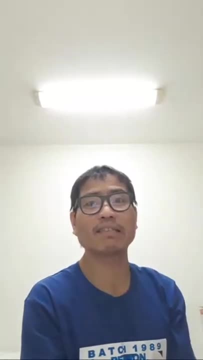 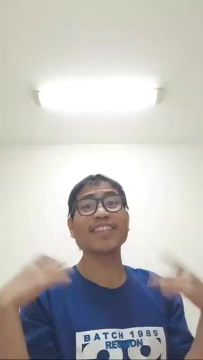 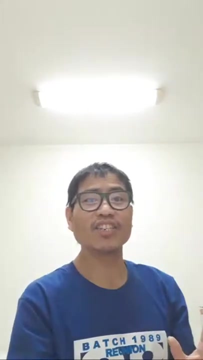 masterpiece and my expertise, expertise, okay, I am more on the organic chemistry or the general chemistry. I am not more on the calculations, because you know, as I said over and over again, I'm not good in mathematics- okay, like that. but I can manage through practice. problem-solving okay, but no, it's not. 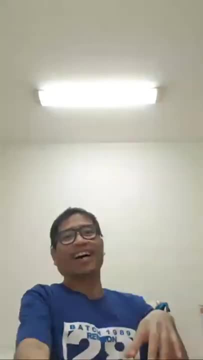 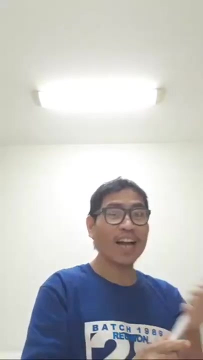 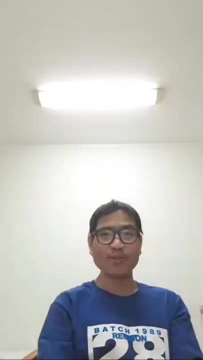 really enough. okay, like that. okay, chemical, you know what I mean. so, chemical reactions, Reaction, engineering- Okay, the word reaction sounds interesting, right? Reaction? Oh my god, You have to interact with people, so there's a reaction behind it. okay, Then, if there is. 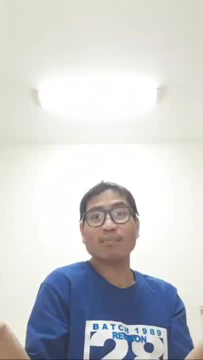 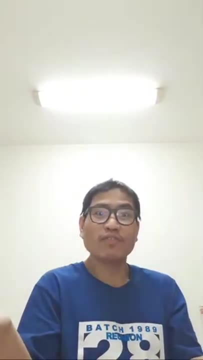 Party A, Party B, Party C, then you have to react between those parties and it's very interesting. Okay then, if you have a girlfriend, if you have a boyfriend, that you have to interact with him also To maintain your relationship- Okay, for a long period of time. 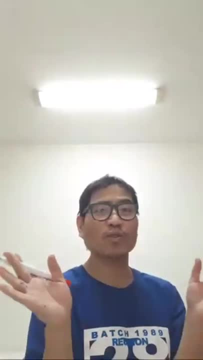 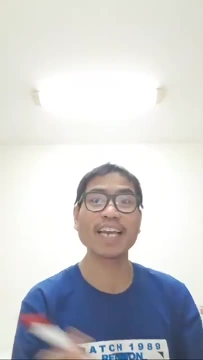 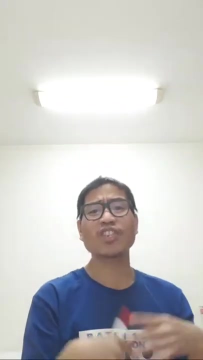 It's just like that, the chemical reaction engineering, and you have also to establish factors that affect those Individual relationship between your boyfriend, between your girlfriend, something like that. So these are also having factors in chemical reaction engineering, for example, the temperature or the pressure, the concentration Right, the catalysts or you know any other factors affecting 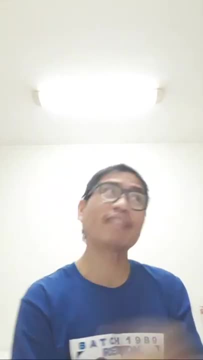 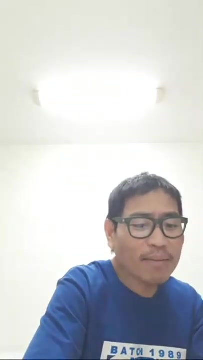 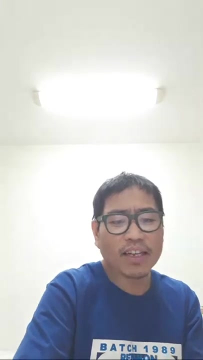 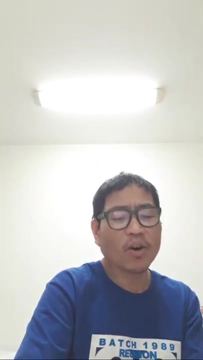 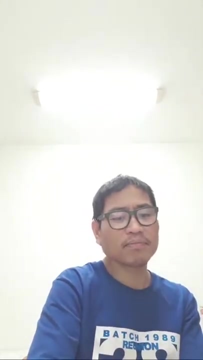 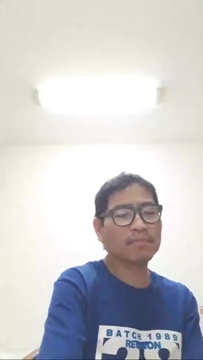 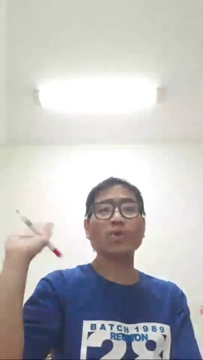 the chemical reaction engineering principles or whatever, Okay, so like that, Okay. chemical reaction engineering: Okay. Or chemical reaction kinetics: Okay. so you're talking about how do you understand chemical reaction and chemical reaction kinetics? Shout out to engineer concordia bacal, so our mentor in chemical reaction engineering, and kevra action kinetics. 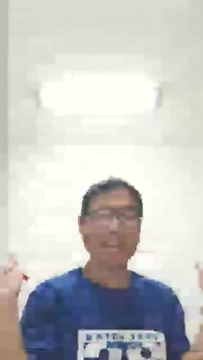 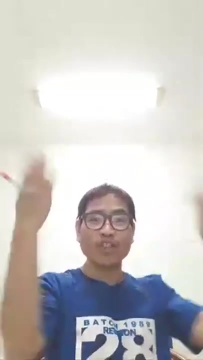 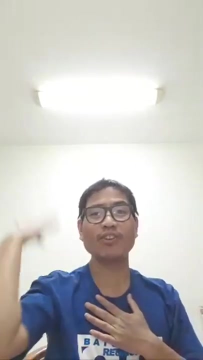 Hi, ma, I'll be able to share information regarding chemical reaction engineering- Cal reaction kinetics. Okay, this is for vlogging on and live streaming only then. if you are watching right now, please correct me also and shout out also to my classmates. engineer timoteo idolantes. engineer ivy at lawan. engineer rio morel. okay, 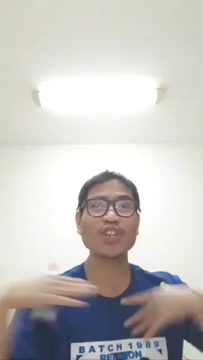 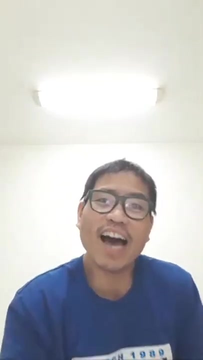 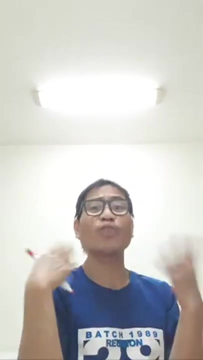 engineer nino chan. okay. engineer stephen flores- oh my gosh. engineer rainier strada. engineer rainier daniella gregory daklan- oh my gosh, please correct me if somewhere along my discussion i have inconsistencies. okay, and also our head of chemical engineering department in cebu institute. 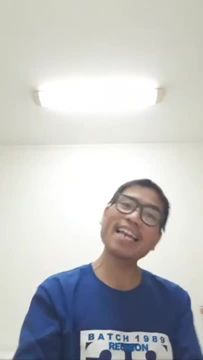 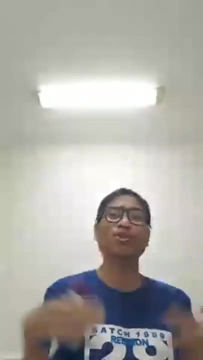 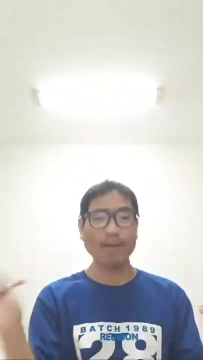 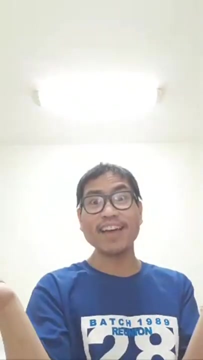 technology university engineer, amis pakamalan. okay, so this is not perfect, but i'll try my very best to explain gradually and smoothly, based only on my little understanding of this main topic: chemical reaction engineering and chemical reaction kinetics. okay, so we'll start now with a data analysis. okay, because, as i told you earlier, this chemical reaction engineering- 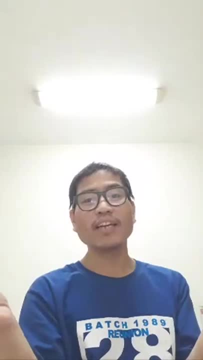 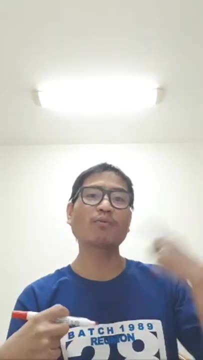 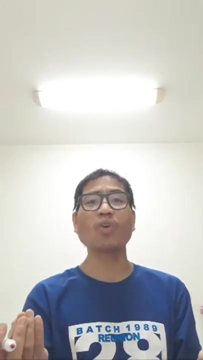 have data, okay, data, to prove your calculations. it's not enough to balance the equation. the number of atoms of the reactant product, the charges, it's not like that. okay, it's always a rate, as i told you a while ago. okay, okay, my gosh. so what is a rate of low, of? 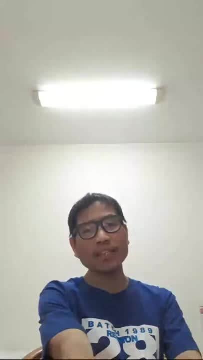 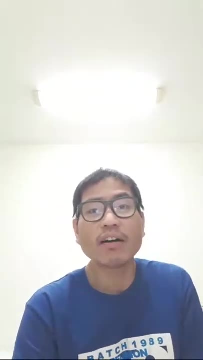 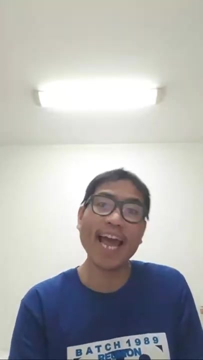 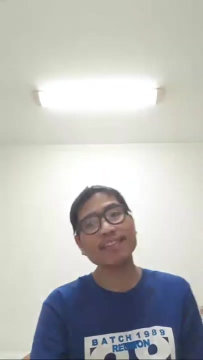 chemical reaction. oh my gosh. so this is basically the equilibrium constant or the rate of equation. constant, okay, multiplied by the concentration a raised to the power, shall we say x, multiplied by concentration b raised to the power, y, something like that. and this, x and y are exponential. 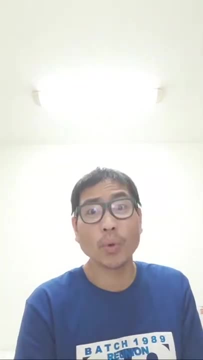 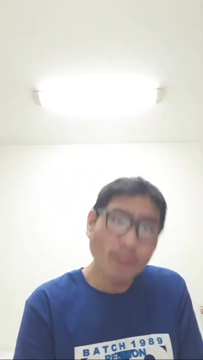 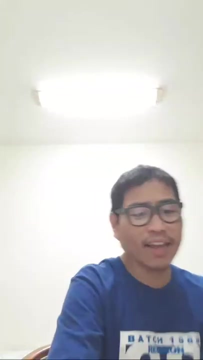 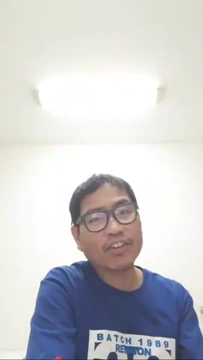 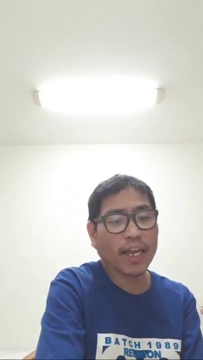 okay, meaning to say this is really, uh, through data in our experiments. okay, so it's gonna be the rate of law of chemical reaction, rate of chemical reaction only. so let's represent that this in way in way. in ways are other textbooks are using small r and other textbooks also are using capital r. it it's up to you. okay, r is equals to k, something like: 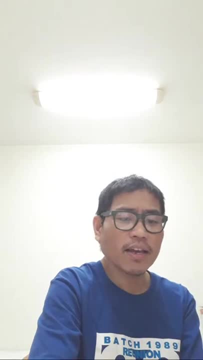 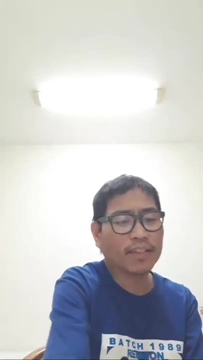 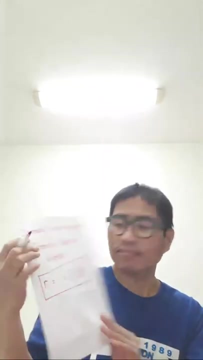 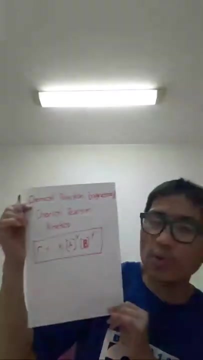 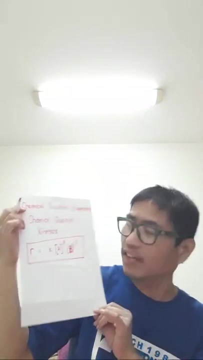 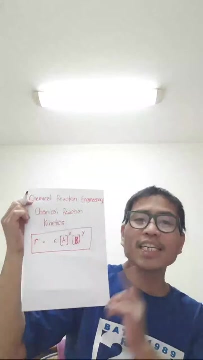 then capital a raised to the power x, y instead of power, sorry- d to the power y. okay, this is our reaction. okay, rate represented as a small r is equal to small k, which is the rate equation, constant, okay. and then times the concentration capital a, rate of concentration capital b, each exponential x. 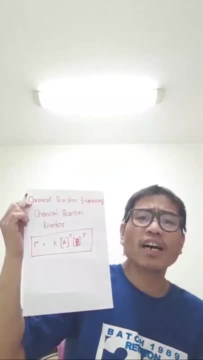 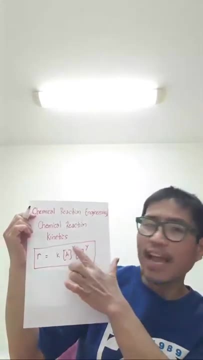 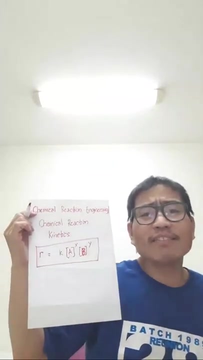 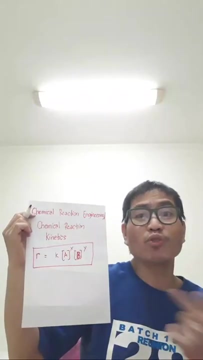 and y, okay, are the order of reaction. okay, reaction order in concentration a is x reaction order and concentration b is y, like that. so if we say what is the reaction order of a? okay, it's the exponent x, it could be one up to nine, it depends on the problem. okay, the same thing. 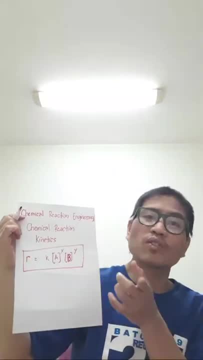 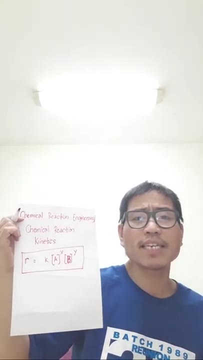 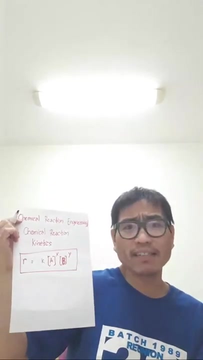 also with the concentration b y is equal to one to nine, it's always b, a numerical figure, a whole number. it should not be a point okay, because it's more complicated to deal with that, though i think having also, but it's avoided to have an appoint something, something like that, okay, so it should. 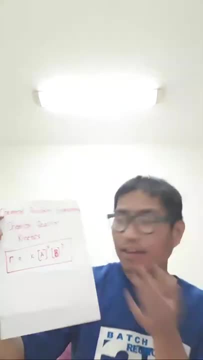 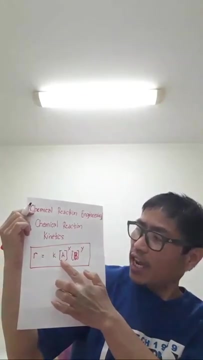 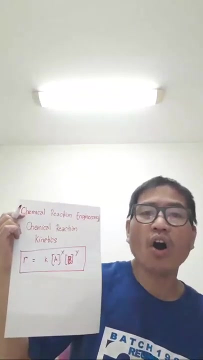 be a whole number, preferably most of the times. i think so. okay, that's the y. so meaning to say that is the reaction order in concentration a: x. reaction order in concentration b: that is y. so we can say now the overall reaction order will be the sum of the reaction. 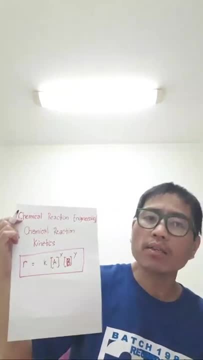 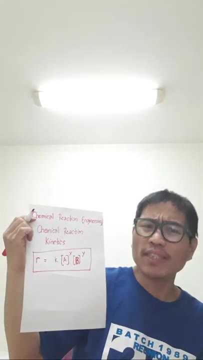 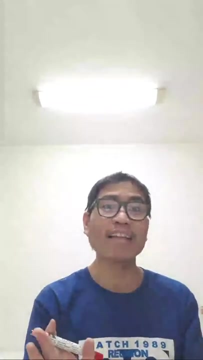 order in concentration a plus the reaction order of concentration b. so that is our overall reaction order, or shall we say small letter n? we will signify or we'll have to denote that as small letter n. okay, don't you worry. n is the number of moles, but in this special topic, 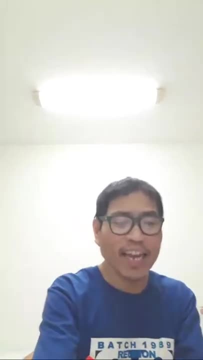 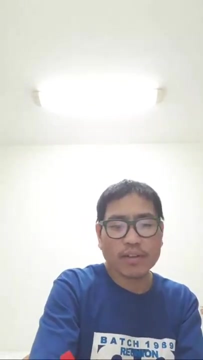 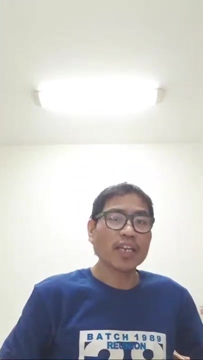 we will be able also to denote that a small letter, n: okay, this is that overall reaction. okay, order, okay, like that. because it's very important also in a problem solving, especially specifically in chemical reaction kinetics or chemical reaction engineering, that the problem will ask you: what is the overall? 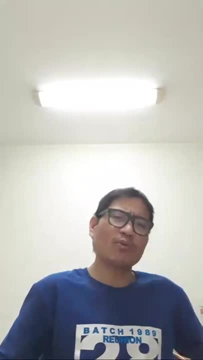 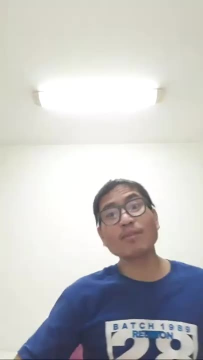 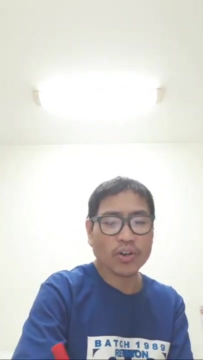 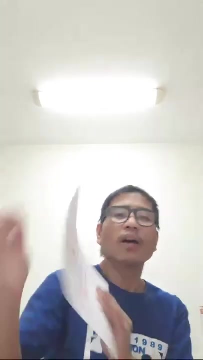 reaction order. okay, what is the reaction order of reaction concentration A, concentration B? then you need to know that. sometimes a question also like that, okay, and then you have to know that also. I just guess that already very clear, right, overall reaction order. okay, like that. okay, now this equation that has an: 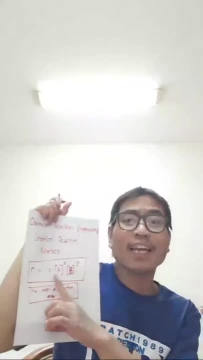 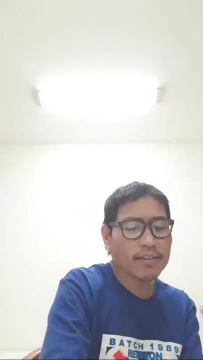 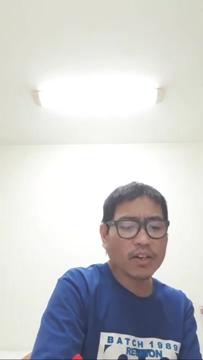 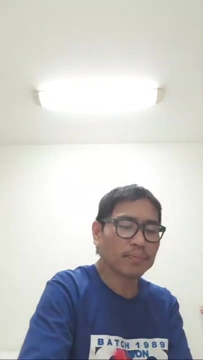 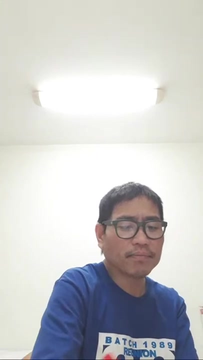 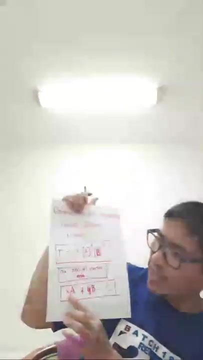 exponential informed. this is derived from the linear equation that goes like this: okay, like this: x times a Plus B, sorry, Y times B is equals to C, Something like that. This one, Okay, Okay. And then algebra right: X times capital A plus okay, Y times B is equals to C. 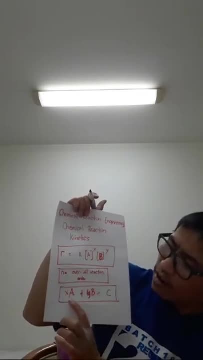 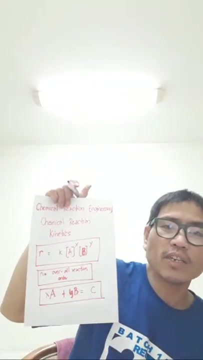 Meaning to say this is: the reaction order X of concentration A plus the reaction order Y of concentration B is equals to C. C is the product. Okay, We denote that as C to make it easier. Okay, Nomenclature only, ha. 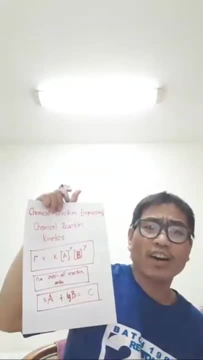 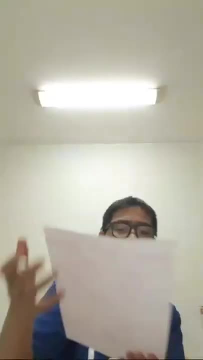 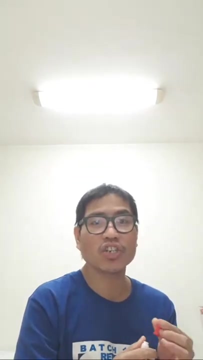 Symbol, or shall we say: only you know an acronym like this to identify easily. Okay, Our formula, Our formula for this. Okay, Like that. So we have also the method of initial rates, That is, a method of determining the reaction orders. 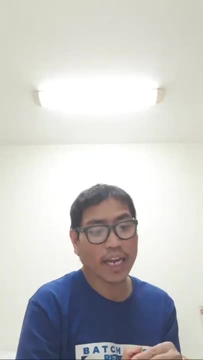 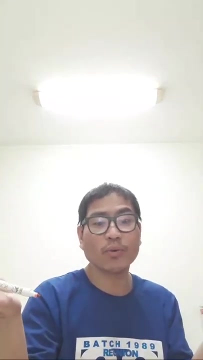 Something like that. So, method of initial rates: Okay, So we have now the overall reaction order. It is the sum of the exponents of the concentration term in the rate of the equation. Okay, Rate equation or rate law of chemical reaction. 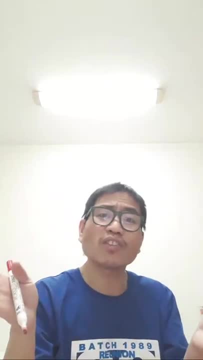 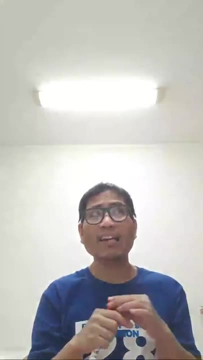 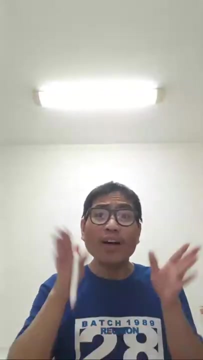 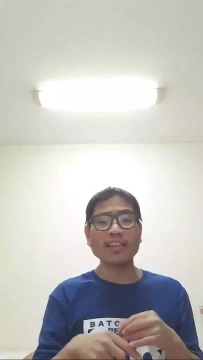 So that's all you have to do, guys, is to master the terminologies, Because we need to use that interchangeably. okay, that's the technique in not only in chemical engineering, also in other engineering disciplines. right, because there are similarities, but the same meaning or the same thing. only don't be confused. if the other terms will be used like that, then you will get lost, something like that, okay. 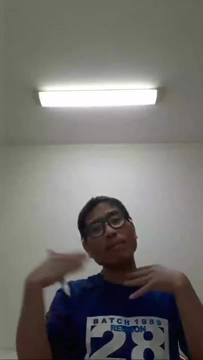 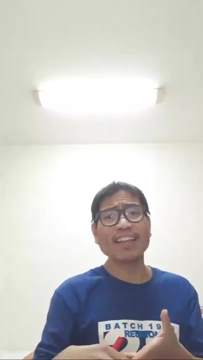 So it's just the same. It could be the rate of law of chemical reaction, rate of chemical reaction, Something like that. Rate equation, chemical reaction. It's just like that, right, As long as we know that that is a small letter, r okay. 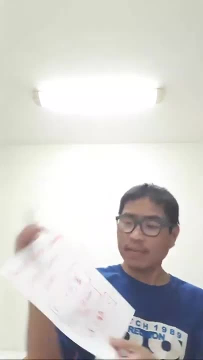 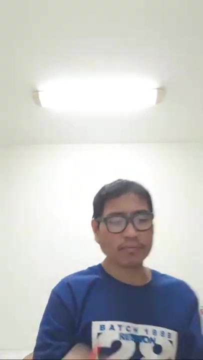 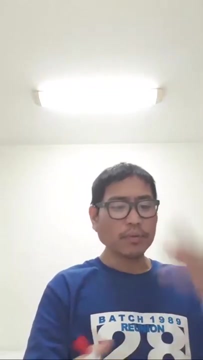 Rate r, something like that, And through this chemical equations we can understand. okay, Like that, Now. okay, We go now to the examples, specific examples: okay, Okay, Okay. Now, for example, I am in the laboratory. 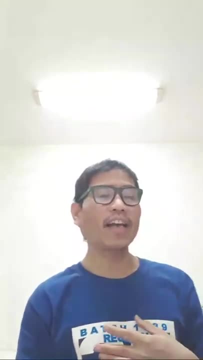 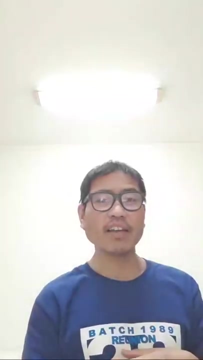 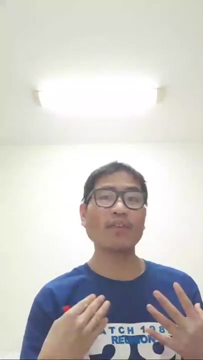 I do analysis, something like that, And I have the concentrations of various you know chemicals. okay, And I prepare that one. okay, I know the concentration in molarity, the most per letter, the rate- Assuming that I know everything- the rate and the concentration, I put that and tabulate that here. 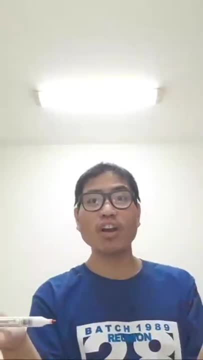 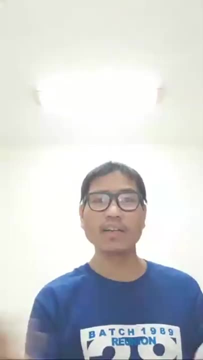 Because this is not a laboratory. This is only verbal explanation to all of you, okay, So this is what I told you a while ago. So many times It's better also to vlog and live stream in actual, inside the laboratory. 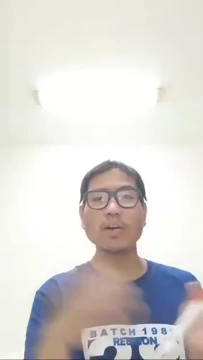 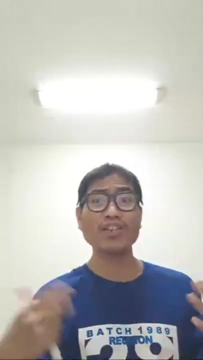 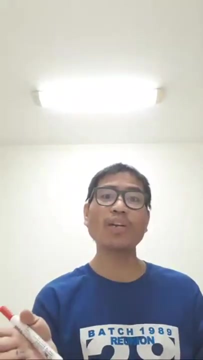 And we should you know so that you can easily understand what I'm talking to. okay, But here it's just only you know an information, a theory, like the basic foundation, the basic knowledge. okay, Sometimes we need to back up with actual applications so that you know it can enhance our knowledge to the specific topic. 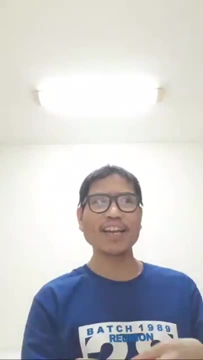 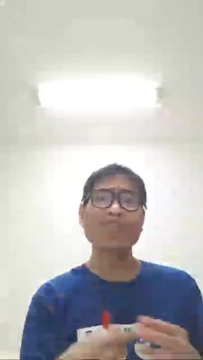 But since I have no time for that, okay, And I don't think so, It's allowed Also when you are working in actual in your company? I don't think so, because that's your personal right. So it could be that you have your own laboratory in your home. 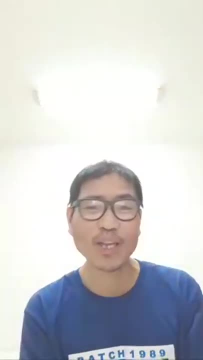 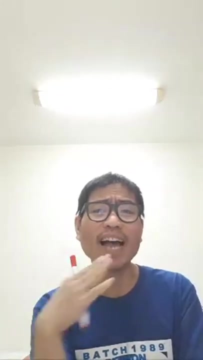 It's okay, I think so In your break time you can do that, But I think it's not also you know approved that you can do that because it's you know it's against the policy of the company you're working with. 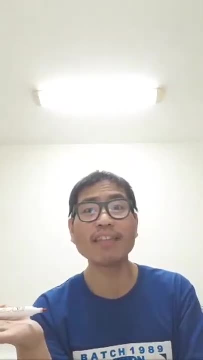 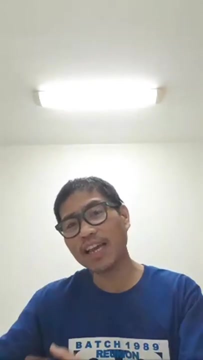 Okay, I think so. Okay, Because that's your personal thing, right? So it's gonna be. Okay, You have your own laboratory to explain that. Okay, You have to do the analysis, the experiments, and you have to discuss properly so that the students can understand. 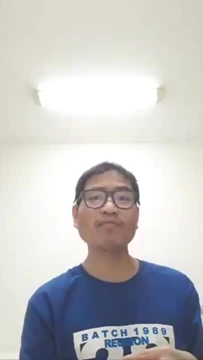 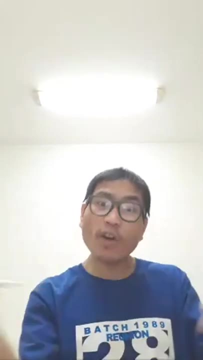 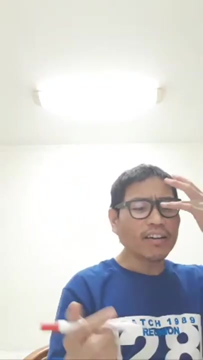 Okay, Theories back up with actual experimentation: Okay, But here only pure discussion and theories. Okay, Like that. But assuming I already obtained the data after my laboratory experimentation, Okay, My gosh. Okay. Now we have, for example, capital M as our molarity. 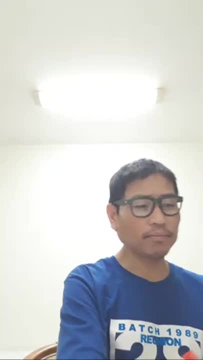 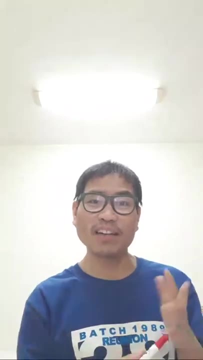 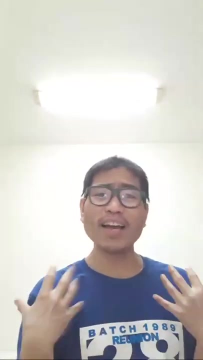 Right Capital. M Like that Gosh This. please correct me, because this is more on algebra. Okay, Algebra, and then a little bit of differential calculus- Okay, But I'm not really that good. Okay, In that kind of you know subjects. 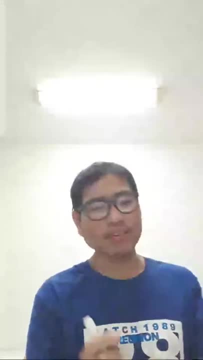 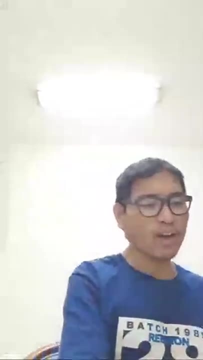 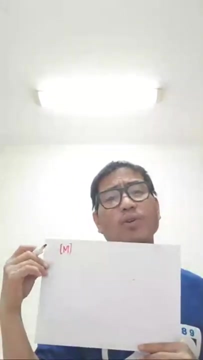 But correct me if I'm wrong. huh, Please, please, please, Okay, Okay, Okay. Uh, Mathematical operation, My gosh And Stance formularity: Okay. Molts of solute per letters of solution. Usually it will be right as capital M directly. 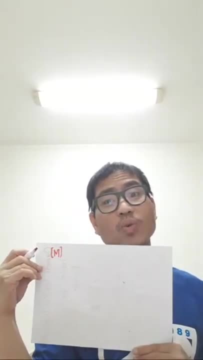 Okay, Especially if you are BS chemistry students, chemical engineering students. No need to you know to state that specifically. it's understood to be a concentration or a solubility. It's a solution with solvent and solute. Okay, Like that. 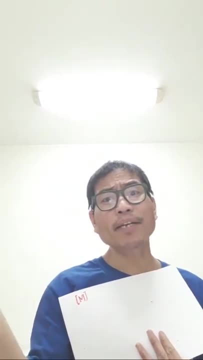 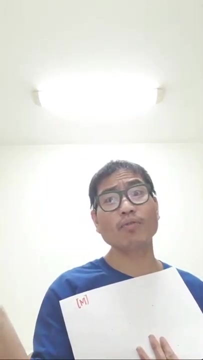 So others also representing a small letter M. But since it will confuse to the molality, Okay, Which is the mols of solute per kilogram of solvent, Something like that, Then you have to write that in a capital M. 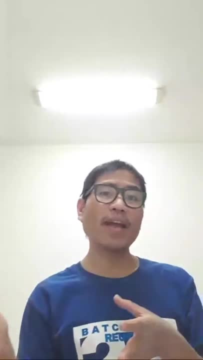 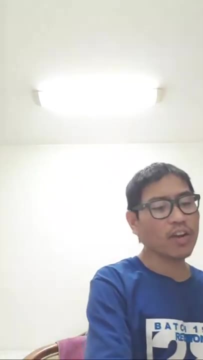 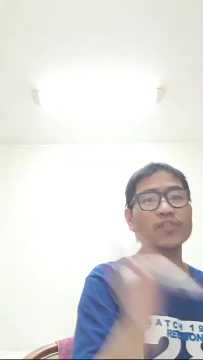 Okay. So, since this is chemical reaction, engineering, so we need to say this: Reaction or concentration, A Okay, Or concentration A Okay, Like that, Okay, Okay. So we start with our first theta One, molar. 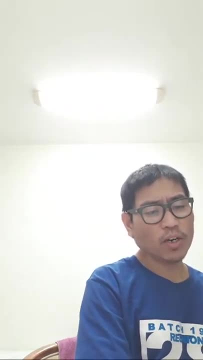 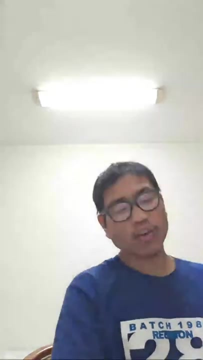 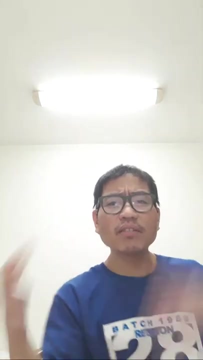 Okay, Then two molar, Three molar, Okay, And then we have our rate, Corresponding rate for this. Okay, You know, actually you should also do the. you know understanding between the capital R and the small letter R. 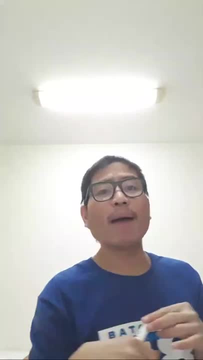 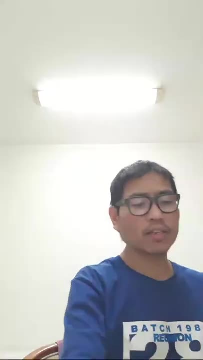 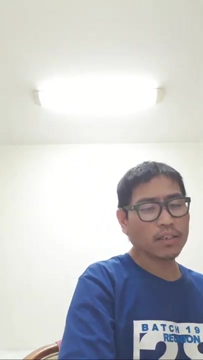 But we should be consistent in our discussion. Since I am using the small letter R for the rate of the reaction, then small letter R. Okay, It could be also capital R, if you want. Okay, This is R. Let's say 0.01,, 0.02,, 0.03.. 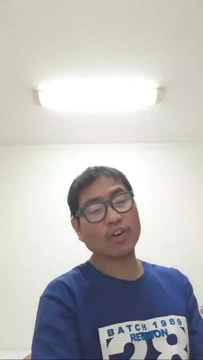 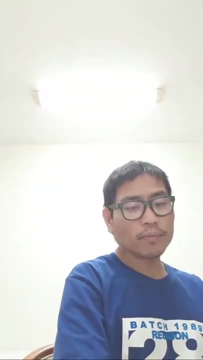 Okay, And this R, as I told you a while ago in my introduction of this discussion that this could be a rate, Okay, So mols, Okay, Mols per seconds, Assuming. Okay, It could be also mols per hour. 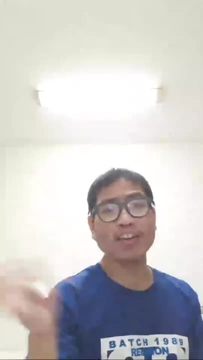 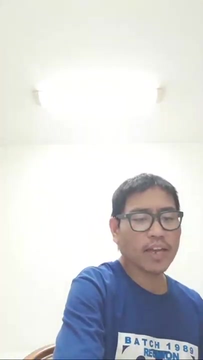 It depends. Mols per minute- Okay, This is only for the sake of basic discussion, Okay. And here is the mols per letter. Okay, Like that. And then we have also another. this is a set of examples. 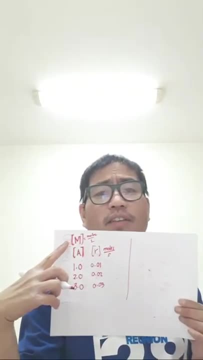 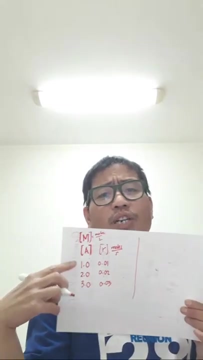 We have the molar capital M. Okay, Represented as concentration A. It's just totally the same Right. So 0.123. In the first experiment. 1.. Second experiment, 2. Second experiment, 3.. 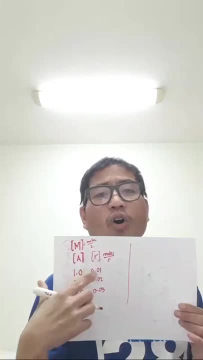 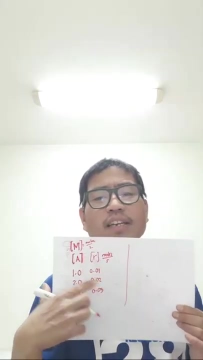 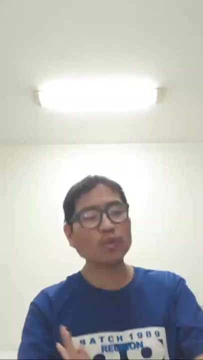 In the first experiment, okay, we obtain a rate of reaction of A which is 0.01.. In the second: 0.02.. 0.03.. Okay, The rest will follow. Okay, Now we go to B, Concentration B, Something like that. 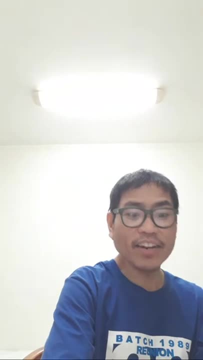 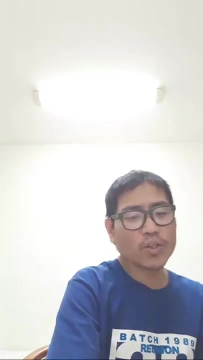 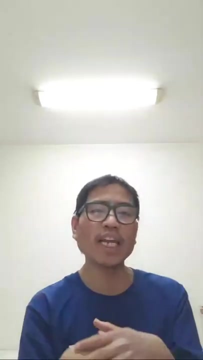 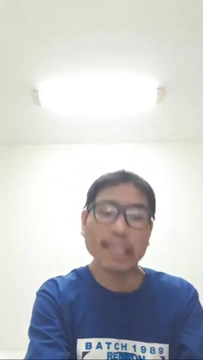 Oh my goodness, Again R, Small letter, R. Okay, It starts with 1.. Okay, 2 molar also And 3 molar. But through the experiments we obtain not similar with concentration A. Our R will be, let's say, example only. 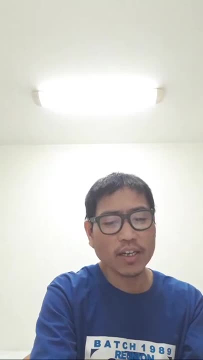 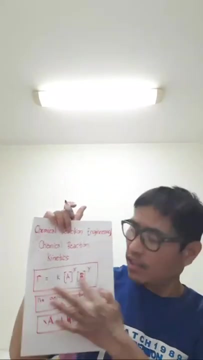 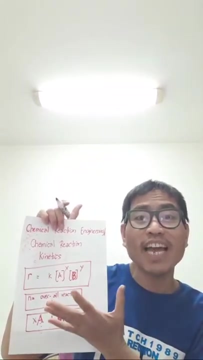 0.01.. 0.03.. 0.04.. And 0.09.. Let's just prove this equation, this one, Why we come up to this. Let's prove, okay, and derive this equation, Why it appears to be like this. 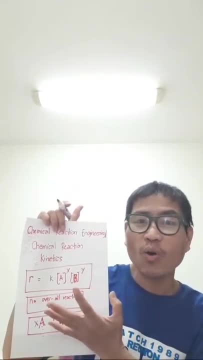 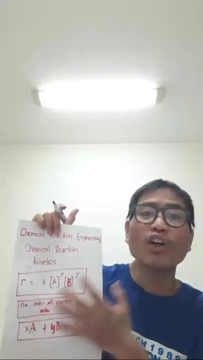 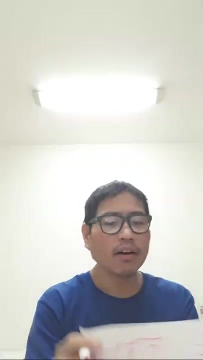 Okay, Where did you get this rate, law of chemical reaction, equation or rate of equation, Okay, Like that. So it should be justified through understanding, through data experimentation, Okay, Something like that. Okay, Okay Now. so we need to. actually, this is more an analysis. 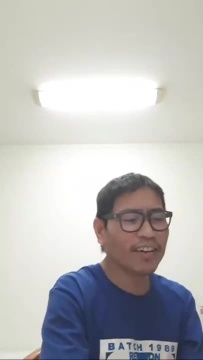 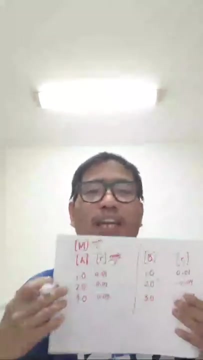 Oh my gosh, Okay, So we have A. So if we increase, take a look, If we increase this by a factor of 2, so this will increase, of course, from 1 to 2, right? 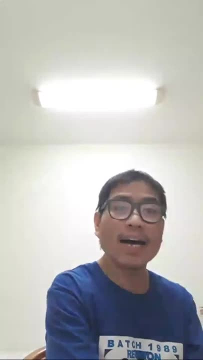 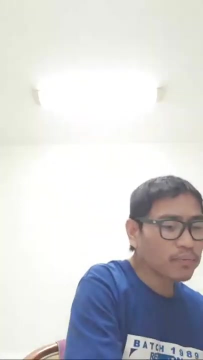 It will increase like that: Arrow up, okay. The same with the oxidation number. The oxidation number. we need to do the arrow up, Blah, blah, blah. Okay, Arrow up, Okay. So 8 increased by 2.. 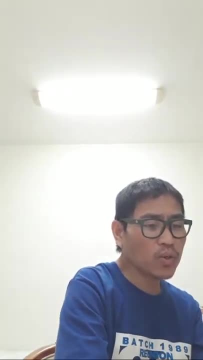 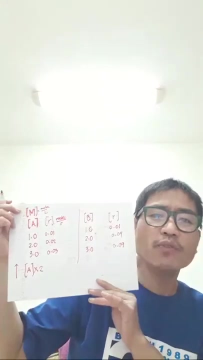 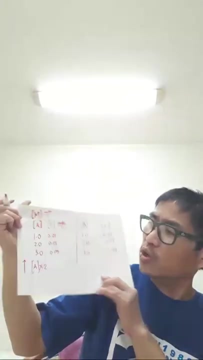 Okay. So if we increase our concentration A by 2, if you take a look also to its corresponding moles per second or rate of concentration, reaction A, so it should also times 2.. Because 0.1, 2.02.. 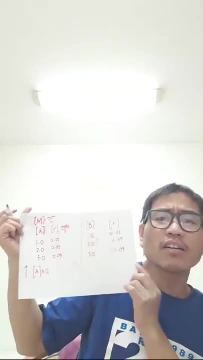 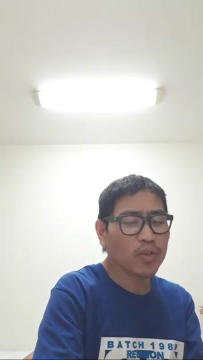 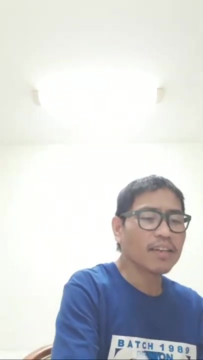 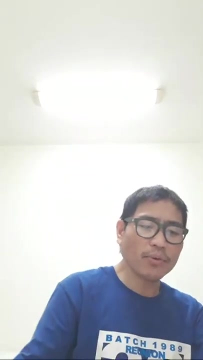 Take the definite: Okay, The difference, Okay, The cap, So it's also times 2.. So small letter, R times 2.. Okay, And then second, Okay, Concentration. A okay increased by 3, because this is also 3.. 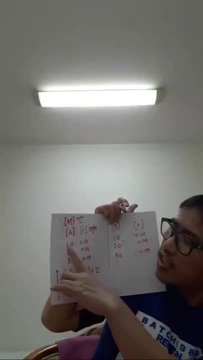 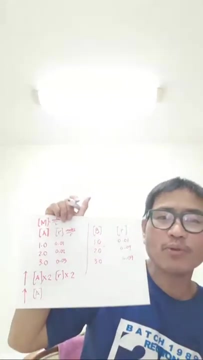 Okay, If you start with the initial okay concentration, then you also go to the concentration A Okay, Then you also go to the final concentration. It's gonna be like that in your chemical reaction: Okay, Initial, final, Initial state, final state. 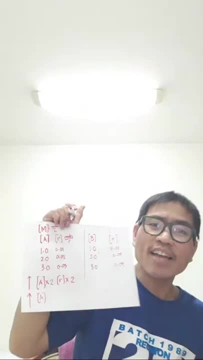 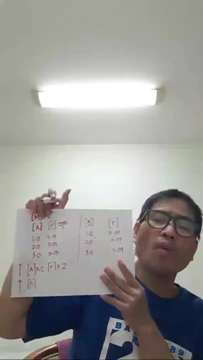 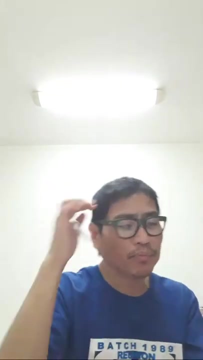 Initial stage, final state, Something like that, So that you can establish an equilibrium concentration reaction which is the basis for low of conservation of energy and low of conservation of matter. Okay In chemistry. Okay, Like that, Like that, Okay. 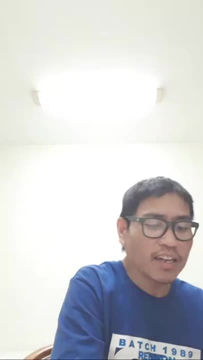 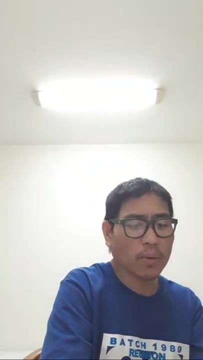 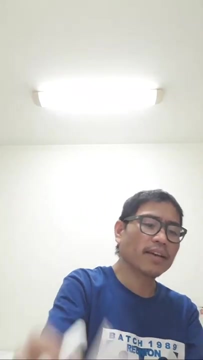 So increased by the factor of 3.. And then small letter R: Okay, By 3 also. Okay, Okay, Okay, Like that, Okay, Okay, Like that, Okay, Okay, Okay, Okay, Okay, Okay. 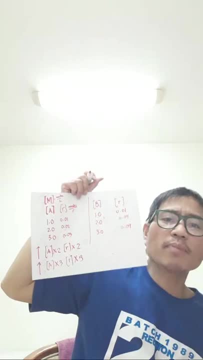 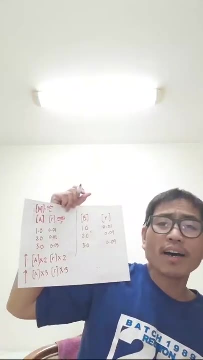 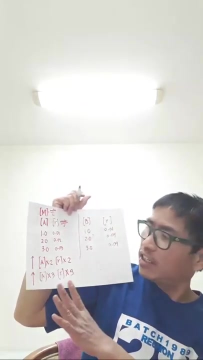 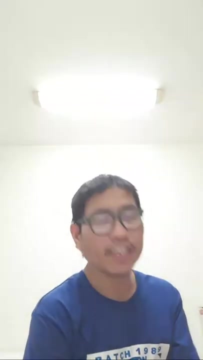 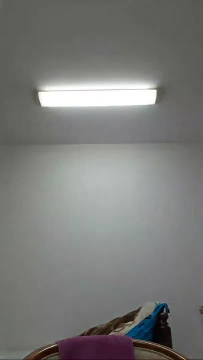 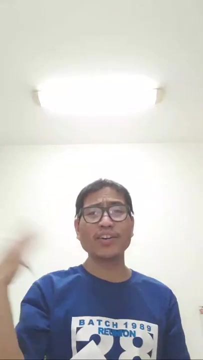 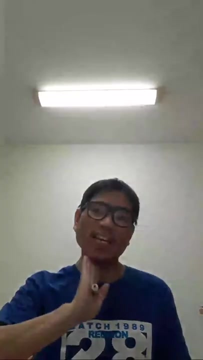 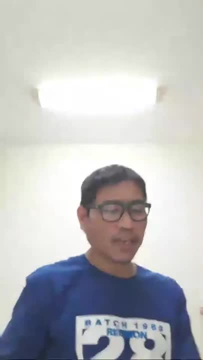 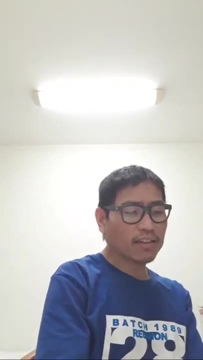 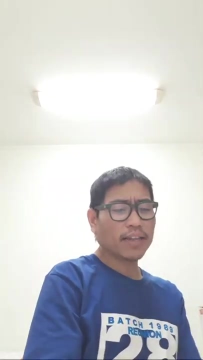 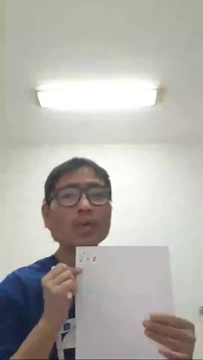 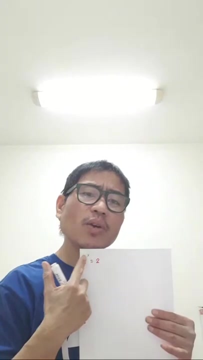 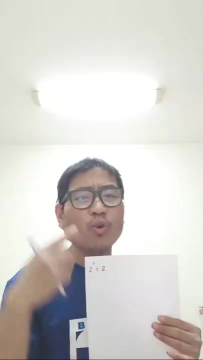 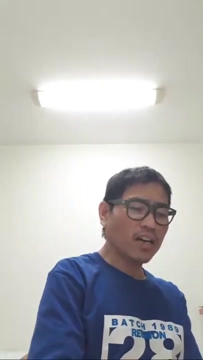 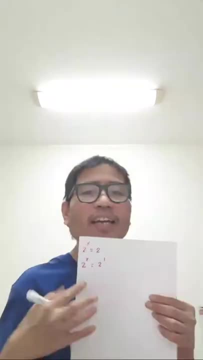 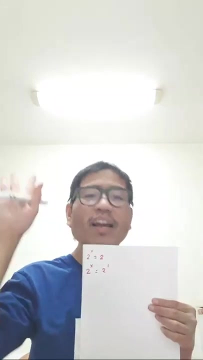 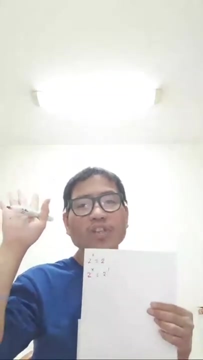 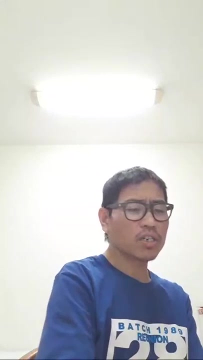 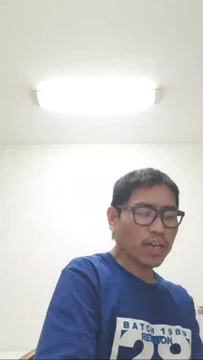 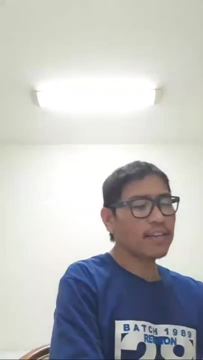 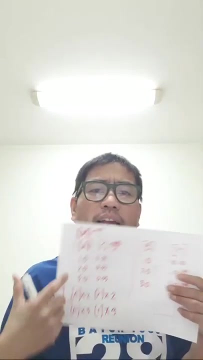 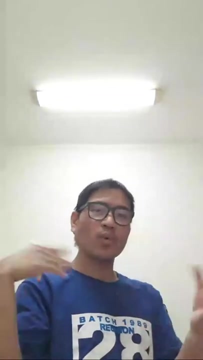 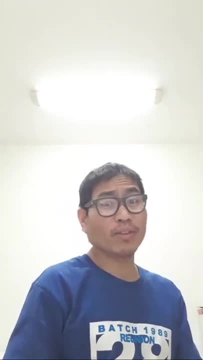 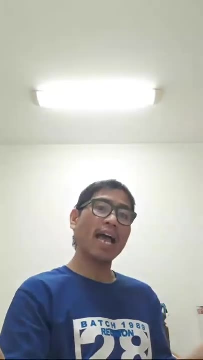 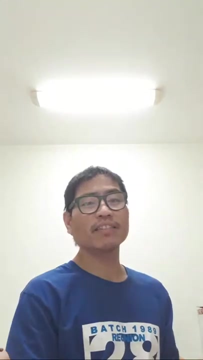 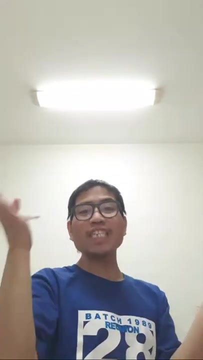 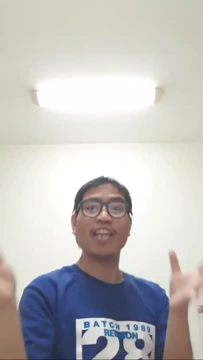 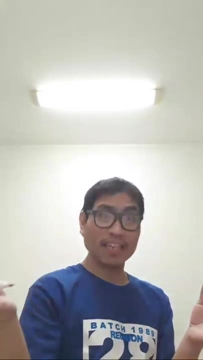 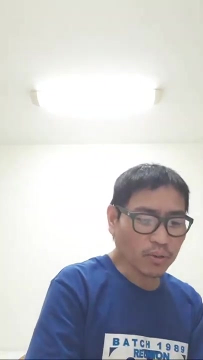 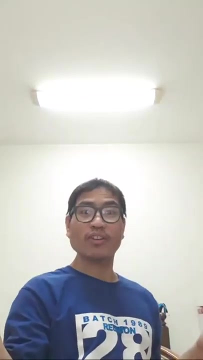 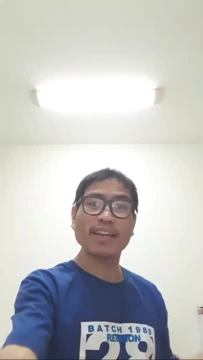 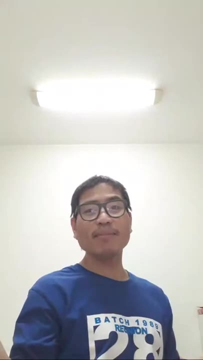 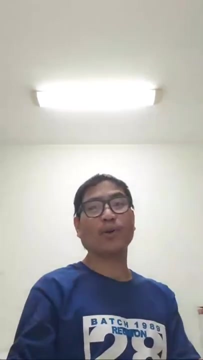 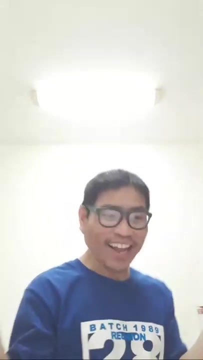 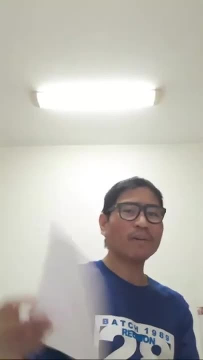 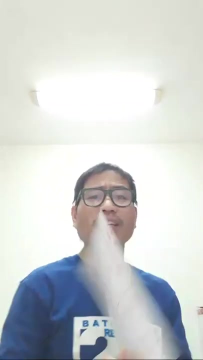 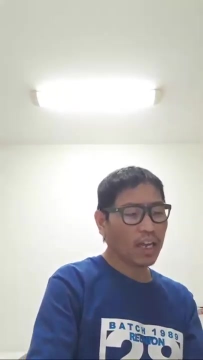 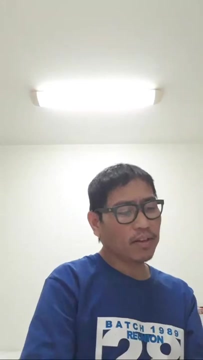 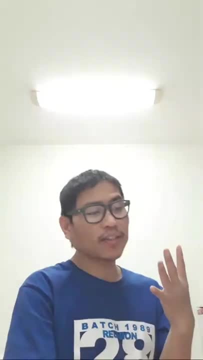 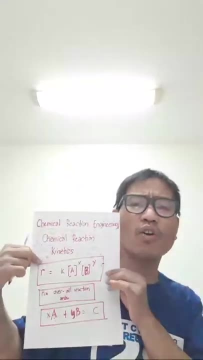 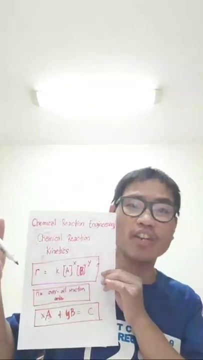 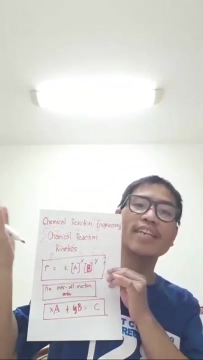 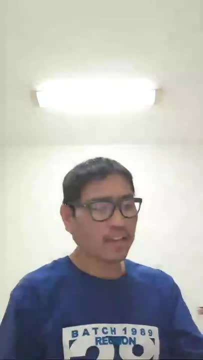 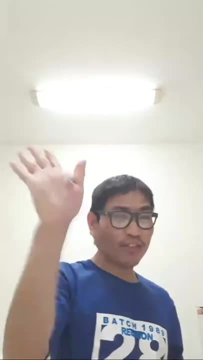 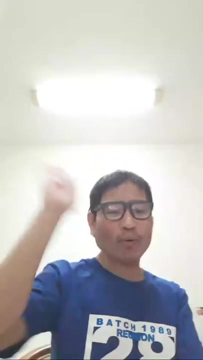 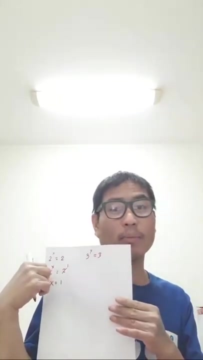 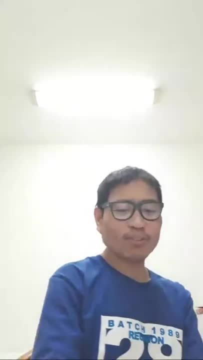 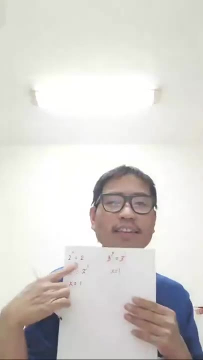 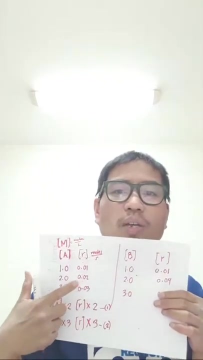 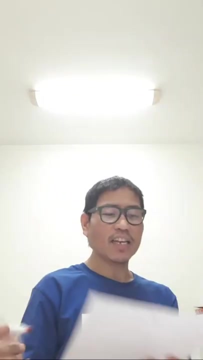 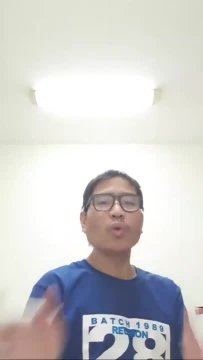 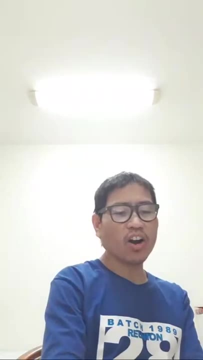 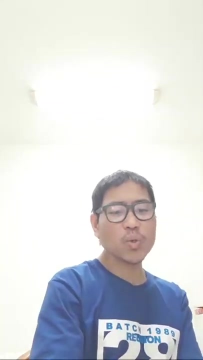 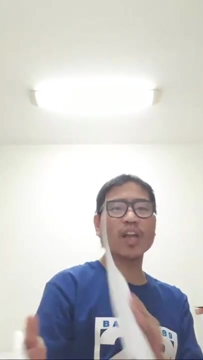 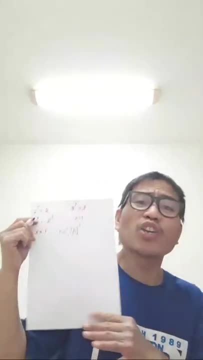 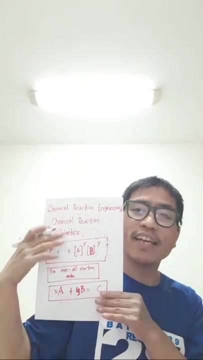 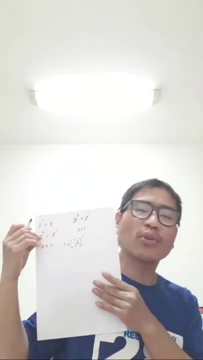 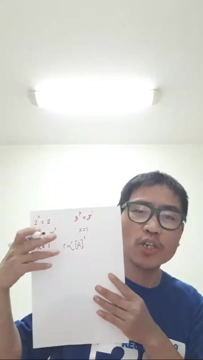 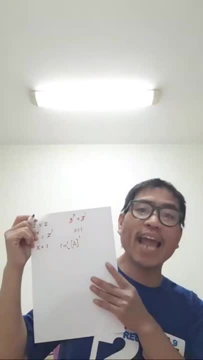 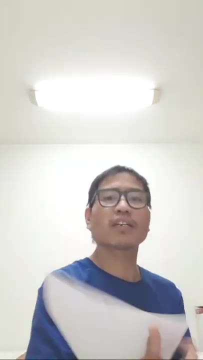 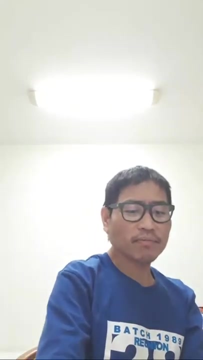 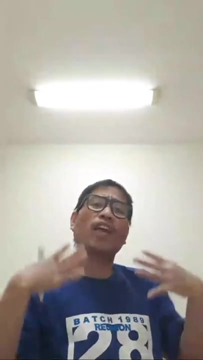 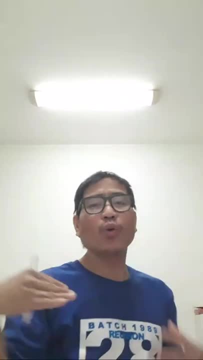 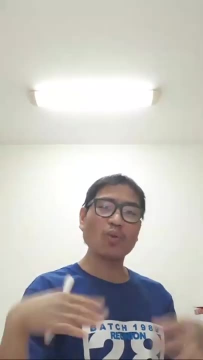 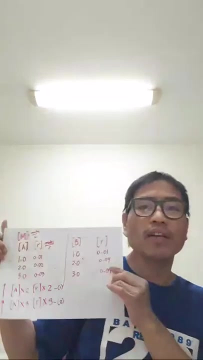 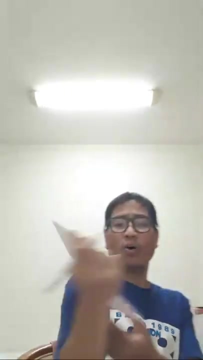 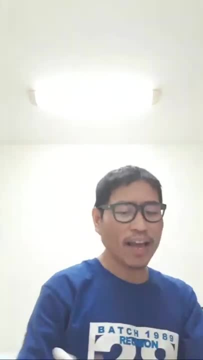 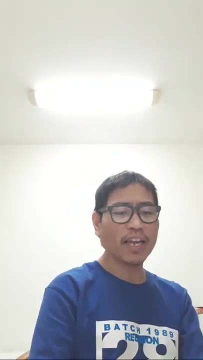 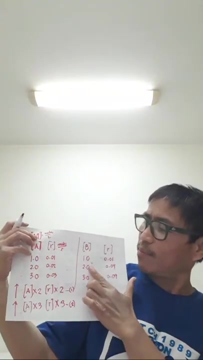 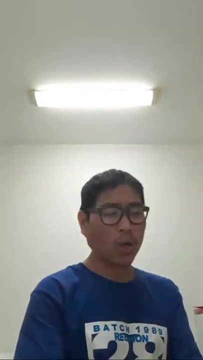 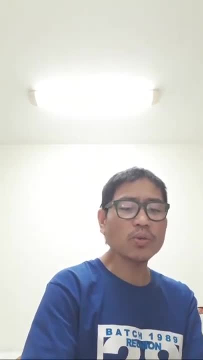 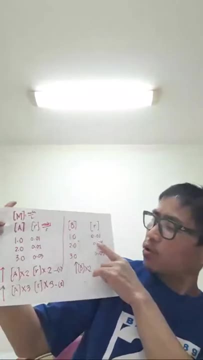 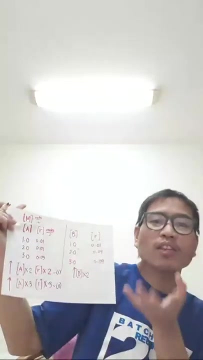 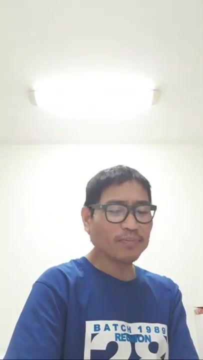 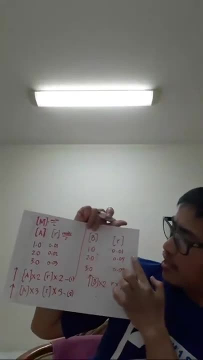 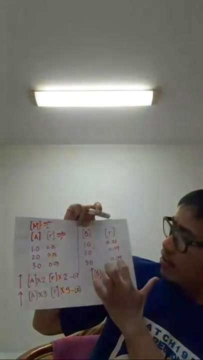 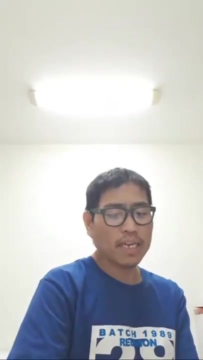 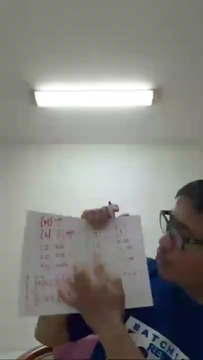 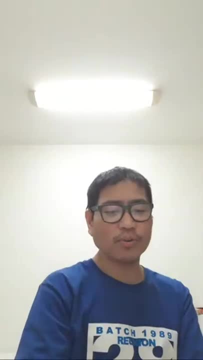 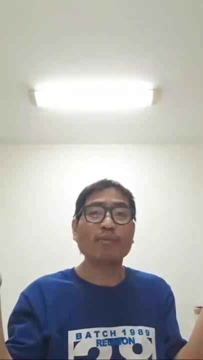 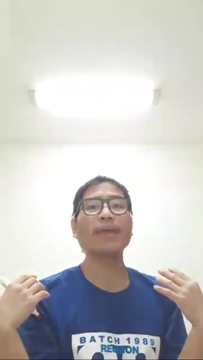 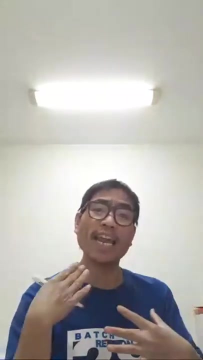 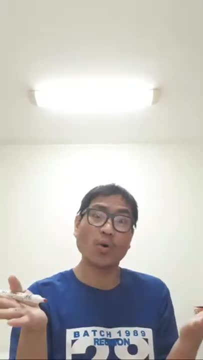 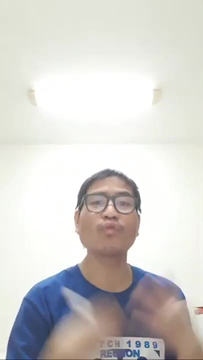 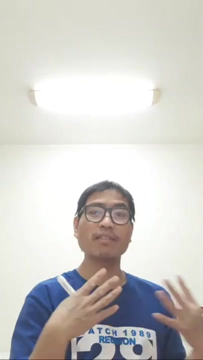 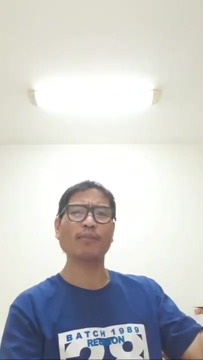 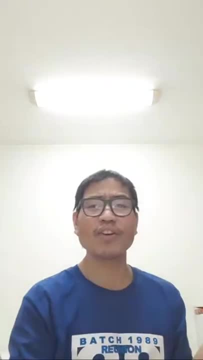 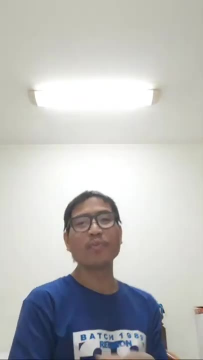 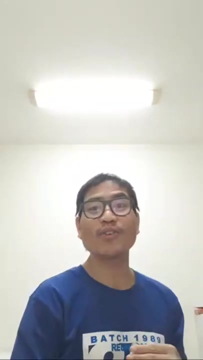 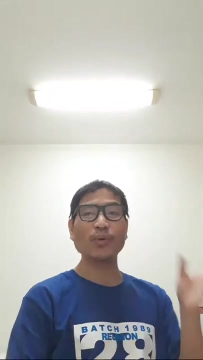 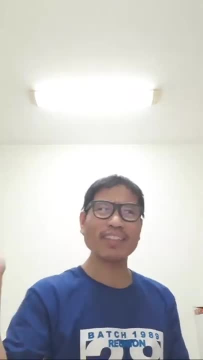 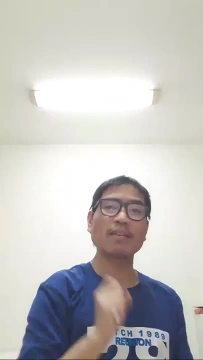 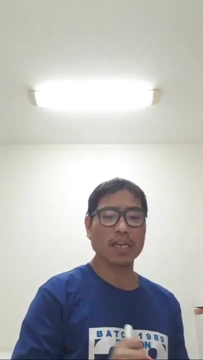 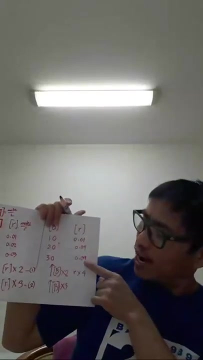 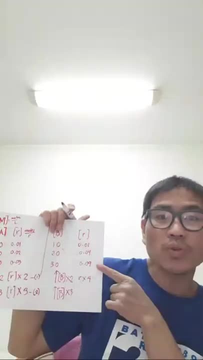 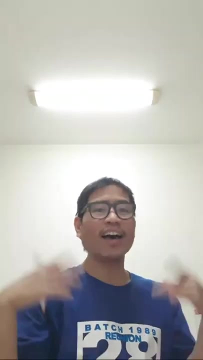 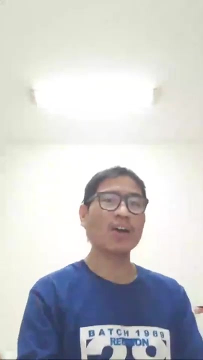 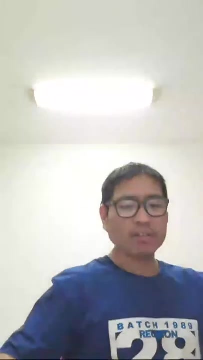 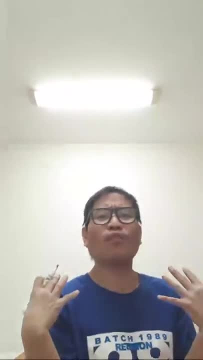 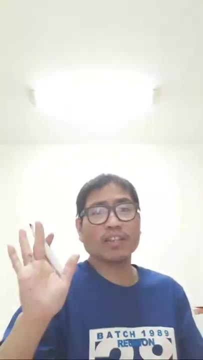 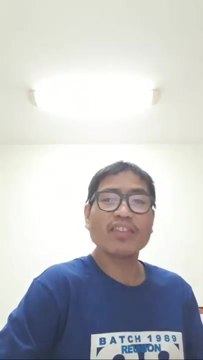 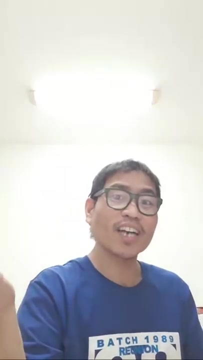 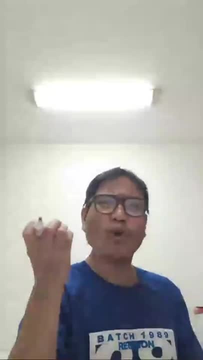 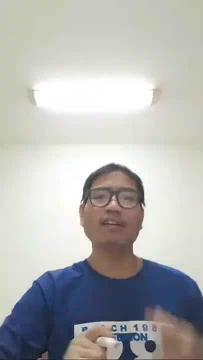 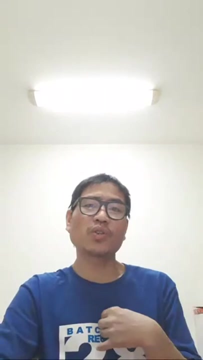 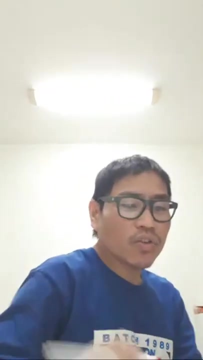 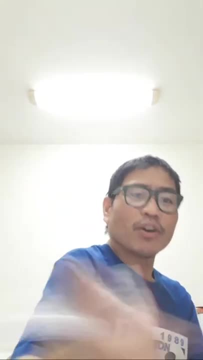 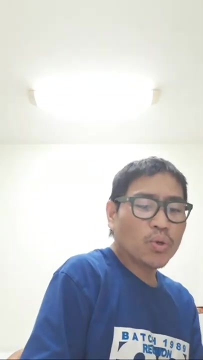 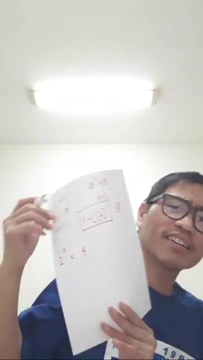 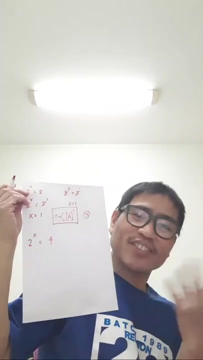 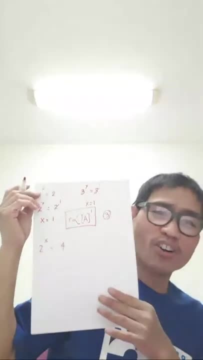 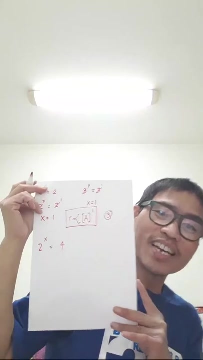 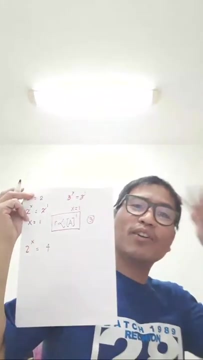 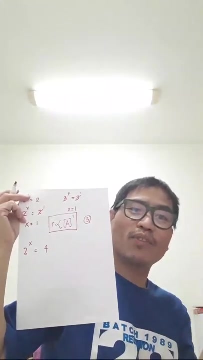 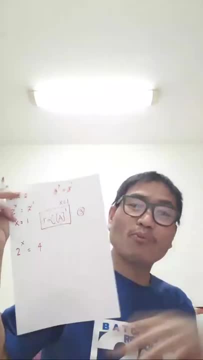 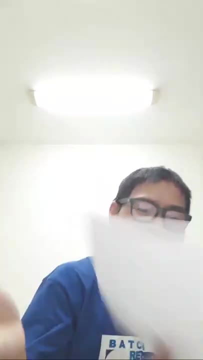 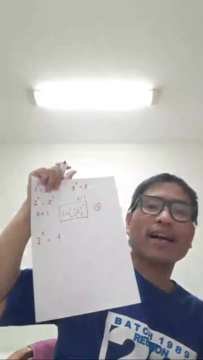 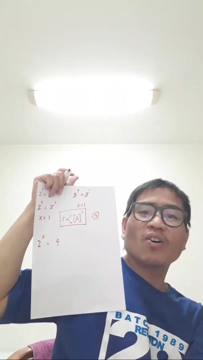 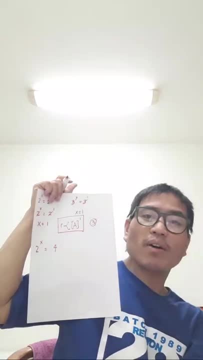 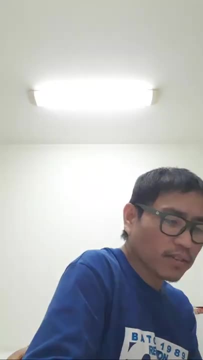 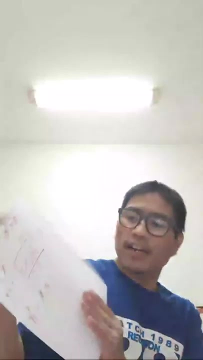 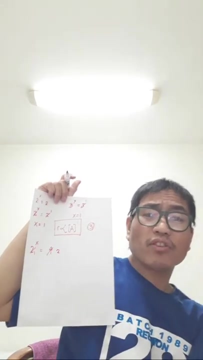 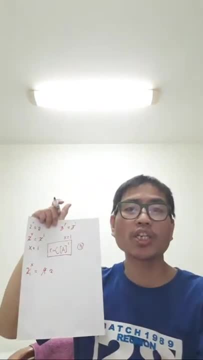 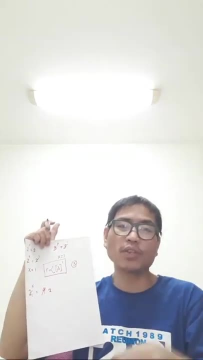 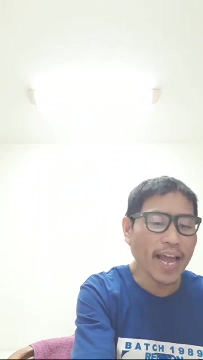 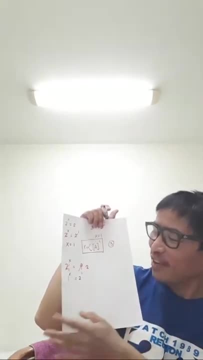 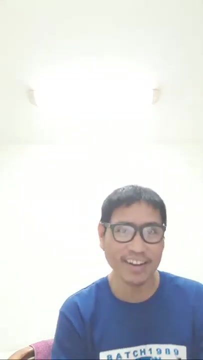 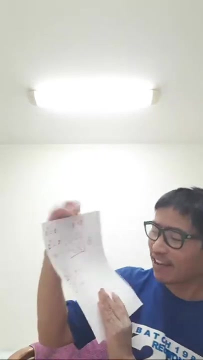 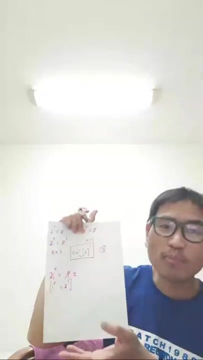 Oh diba, Okay, like this Now. oh my gosh, the x is in the exponent Again, algebra. Okay, This will be multiplied both by 1 over x to cancel the x here on the left, And both should be multiplied okay. 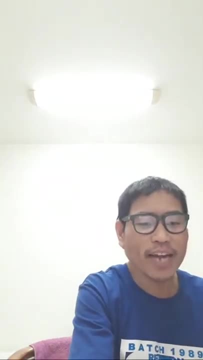 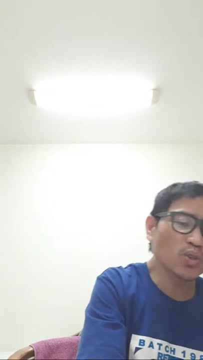 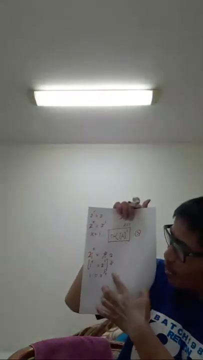 Of course. So if multiplied by 1 over x, it will be cancel the x, so it will equal 1 on the left side. And then we have 2, 1 over x. Oh my gosh, 1 is equals to 2 over raised to the power of 1 over x. exponential or fraction. 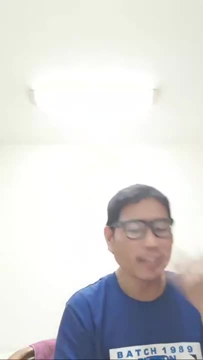 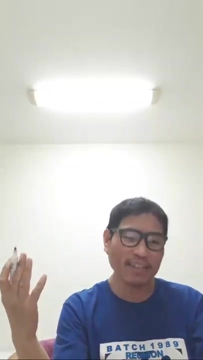 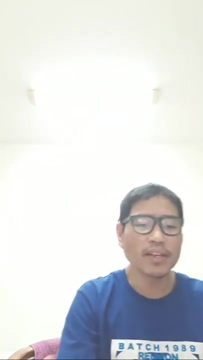 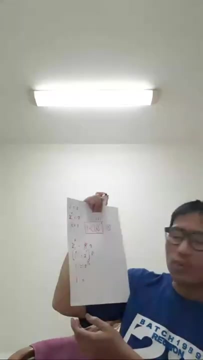 We're here again, Okay Now. okay, so we need to break down to solve the value of x. Okay, Okay, 1 is equals to this. x also can be written as: okay, x squared, So x squared of 2, okay, because this is also the same as 1 half. 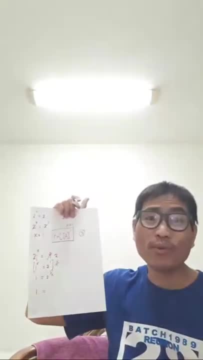 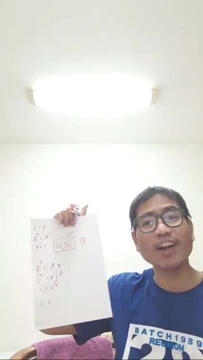 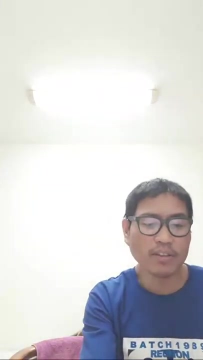 When you raise the number to 1 half. that's square root right. But that's the basis not only to numerical figure fraction but also to involve variable. That principle will be applied also. So you have to do this: x squared of 2.. 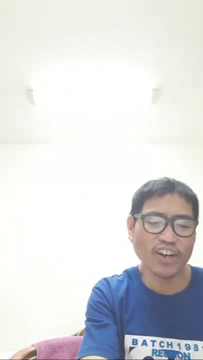 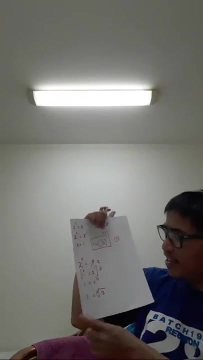 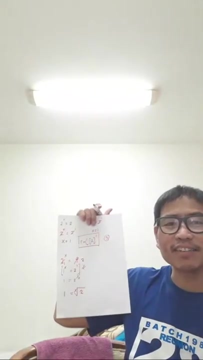 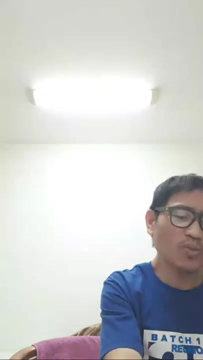 Oh my gosh, Ganon. So x squared of 2,. right, Now again. multiply this both sides with 2 to cancel the square root. What will remain is the x, See Kanon ka. Okay, 2, 2, then 1 to the power of 2 is equals to 2x already. 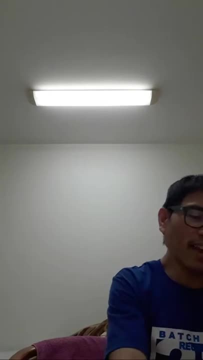 Like that. okay, Okay, 2x, cancel and 2,, 2,. okay, Like that. Okay, So 2 to the 2x. Okay, Like that. So this is 4x and 1.. 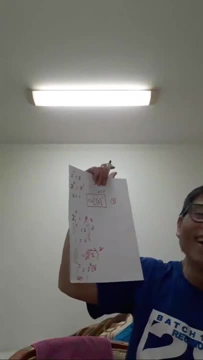 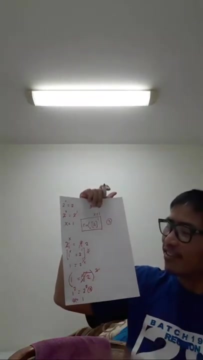 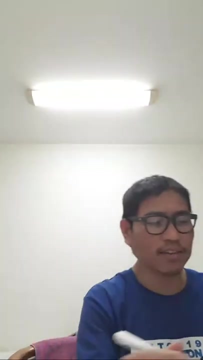 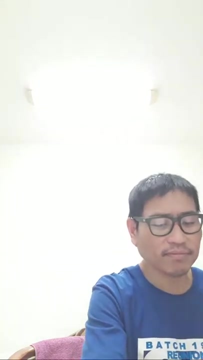 Okay, Like this. Okay, Take that as a reaction, because this will not be canceled. That's why that's the story behind: Okay, Like that. Okay, Now solve for the value of x. Okay, Okay, So. 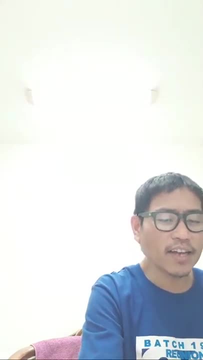 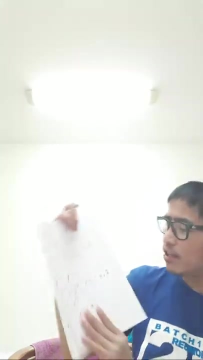 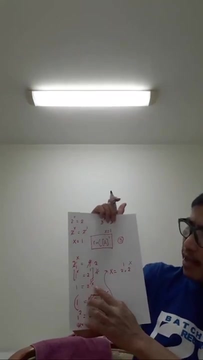 2, 1 times 2x. Okay, Like this, 2, 1 and 2x is 1.. Because in algebra you have to. for example, this is xmn. You remember that one in algebra? 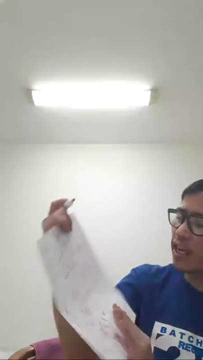 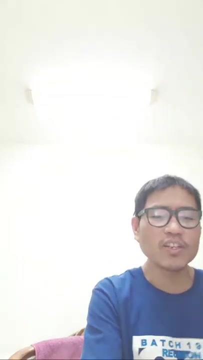 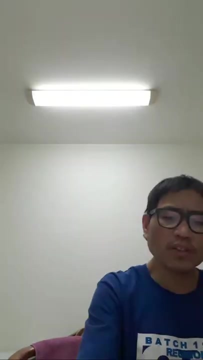 If this is xmn, you have also to say xm and xn. right, Okay, So like that. So this is okay. So 2, 2x, x, 2, 1- cancel. So this becomes our x. 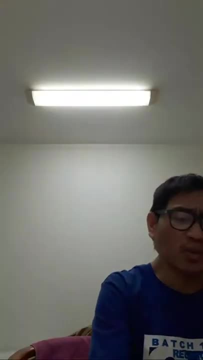 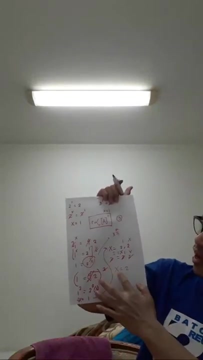 Okay, And this is x, 2, 2.. Okay, So cancel also 2.. So x is equal to 2.. This one, Okay. so x is equal to 2.. Okay, Go over to this equation and solve by yourself. 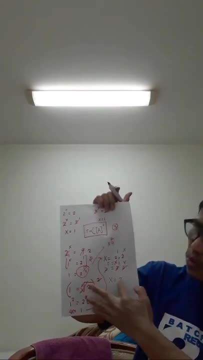 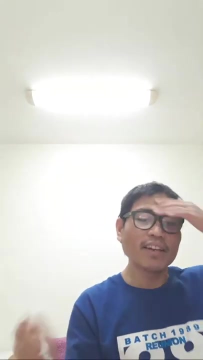 We can obtain the same like this: x is equal to 2.. Okay, You understand now Algebra, Anyway. also, I'm confused a little bit, But you know, just govern with this: x raised to the power, m and n, like this: 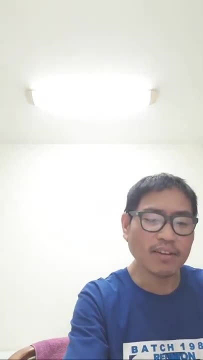 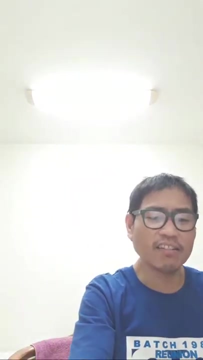 And then the other side also will be like this: Okay, 1 raised to the power. like this: Okay And x. I'm going to solve. Okay, Since x is equal to 2.. Okay, So x is equal to 2.. 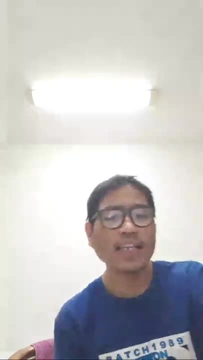 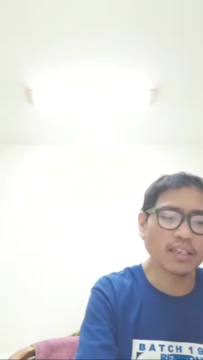 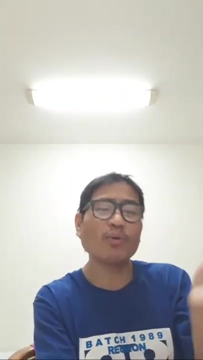 Something like that: Okay, And the other one here: b, Okay, b to the y, Okay, y. Actually it's just the same principle, But I forgot that this is already y, Okay, But actually, what in my mind is just the same? 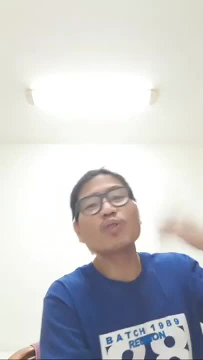 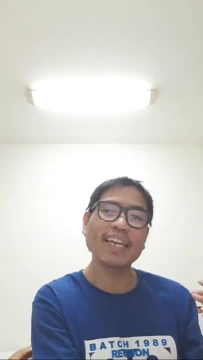 It's just the same reaction order Only. the difference only is we need to use another variable. Okay, The principle is still correct, But the variable we choose is not really different. Actually, we need to use another variable. Sorry for that. 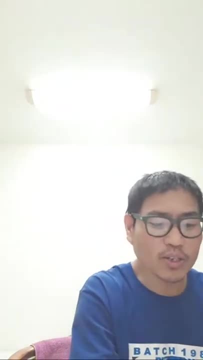 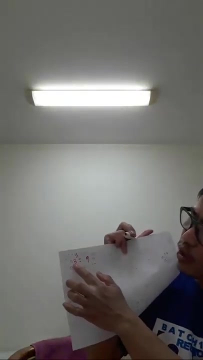 The principle is just the same. Now to complete: Okay, 3y is equal to 9.. So, in order to make this 9.. So we need to multiply this by 2.. 2 itself, That is 3 times 3, is equal to 9.. 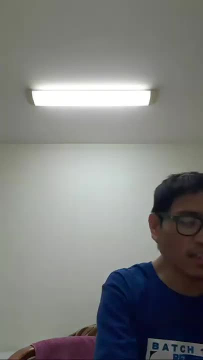 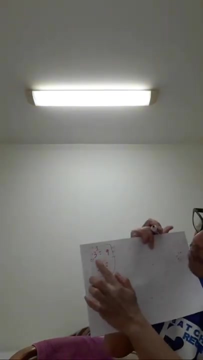 Okay, So y is equal to 3.. Oh, 2.. Sorry, This is an equation Okay. 3 raised to the power of y, Equal to 9.. So, in order to get 9,, you have 2 times 3.. 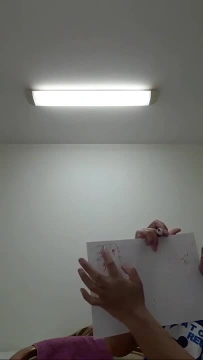 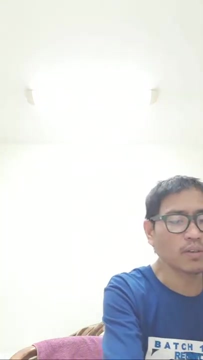 This: 3. Exponential 2.. So 3 times 3 is equal to 7. It will be equal. So y is equal to 2.. Now we have now: y is equal to 2.. Okay. 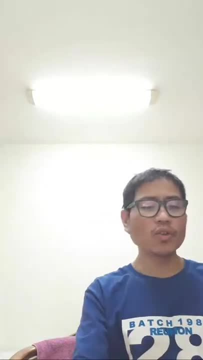 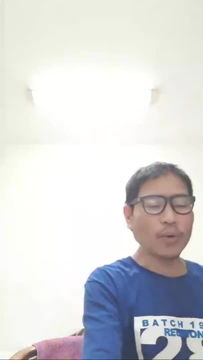 Like that. So we need now to substitute that 1 in our rate-load equation, Like that. Okay, So we have now the rate in our general equation here. Where's that 1? This 1.. This 1.. 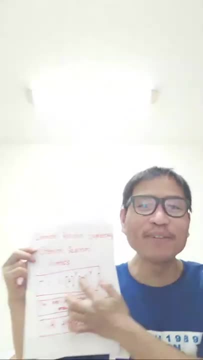 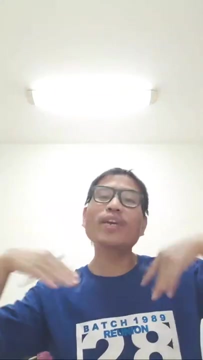 Oh my gosh This. 1. Use this 1, huh, Okay, But actually we will correlate that. 2. The concentration A and concentration B, with its corresponding rate of reaction A and B. Okay, Now this 1.. 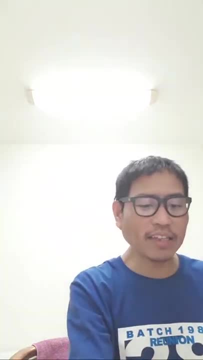 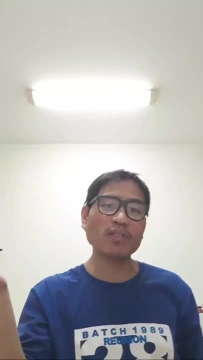 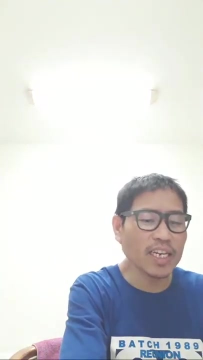 Okay, Now be careful. So rate is equal to. Actually, some books go directly with a constant, But I have to explain also why the constant will appear. Okay, So like this. Actually, this is Rate Key. 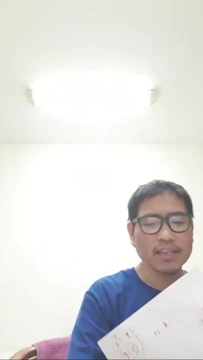 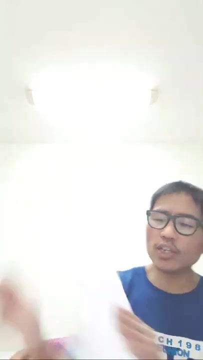 We need to combine the 2., The A and B. Okay, So it will become now: Concentration of A raised to the power 1., Which is the value of x is equal to 1.. We solved already. And then that's the concentration B. 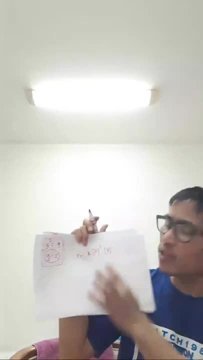 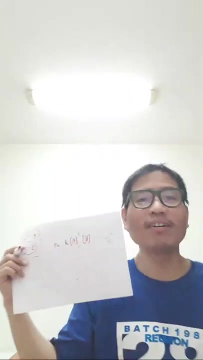 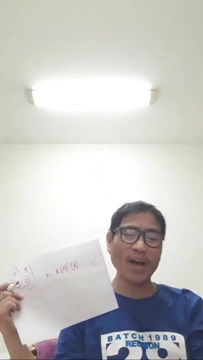 Which is the y equal to 2.. We solved already, It's here, Right. There's no whiteboard, So it's a bit confusing. So my discussion is very, you know, turbulent Because I don't have the whiteboard and any, you know animation to make my discussion very clear. 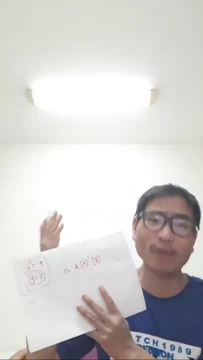 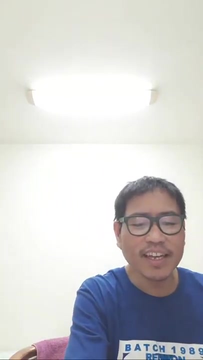 But don't you worry, The foundation is in my brain. Okay, That I have to just share with you. Okay, Like this. This goes to 2.. Like this, So R? Putting 1 as an exponential is the same as don't put that 1.. 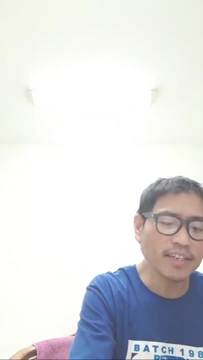 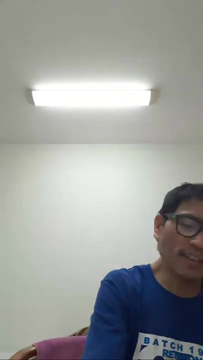 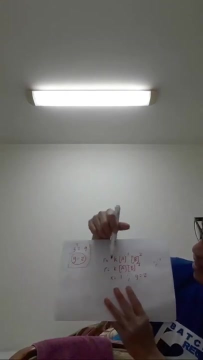 That's in chemistry. Okay. So K, K, A, B, 2. And x is equal to 1. And y is equal to 2.. Okay, This one. Okay. So R is equal to K times A, raised to the power 1.. 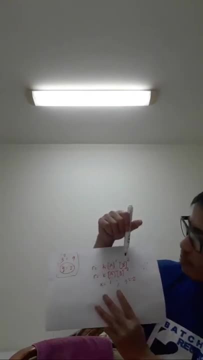 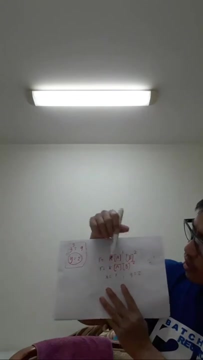 Based on the data experimentation, we obtained Times concentration B raised to the power 2.. So K is equal to A times B raised to the power 2.. In which our x is equal to 1. Or y is equal to 2.. 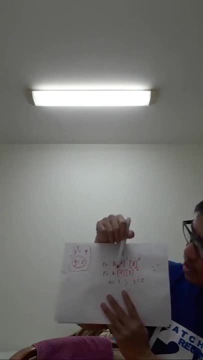 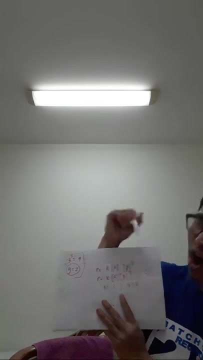 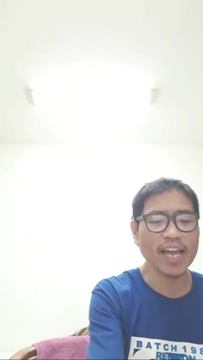 So this x is the reaction order in concentration A. This exponent Y is the reaction order of concentration B. So the overall reaction order 1 plus 2 is equal to 3.. Or something like that. So N is equal to x plus Y. 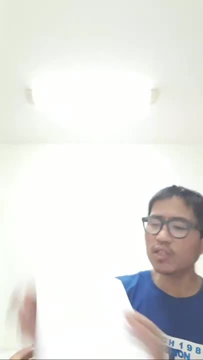 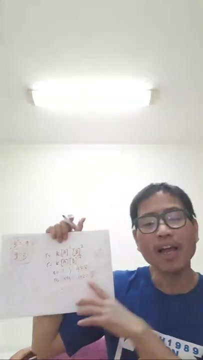 So 1 plus 2 is equal to 3.. If the question was saying in the problem solving: What is the overall reaction, What is the reaction order, So your answer will be 3.. What is the reaction order of your concentration? A? 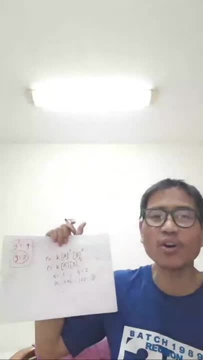 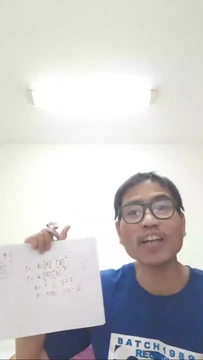 So that is: 1. What is the reaction order of concentration B, That is, 2. In which these numbers? we solve that through algebra In the series of experimentation data that we gathered inside the laboratory, Something like that. Okay, All you have to do is to you know. 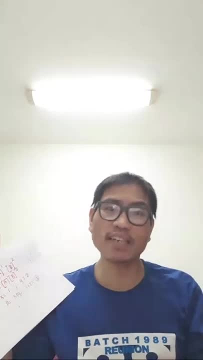 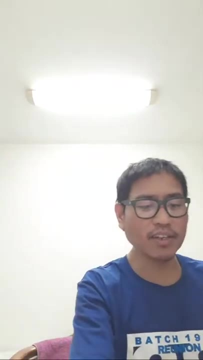 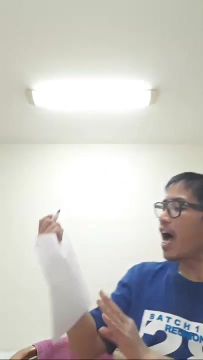 Is to, you know, Incorporate algebra in our brain Somewhere in our discussion And communicate that Properly to your discussion. Something like that, Okay, Like this, Okay Now. Actually, the K should also be denoted as: 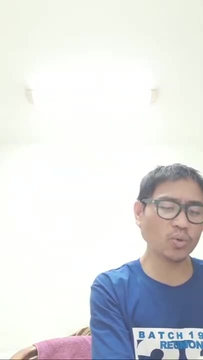 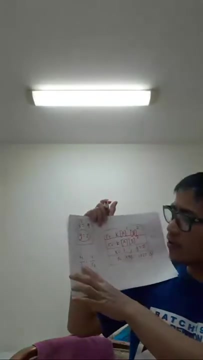 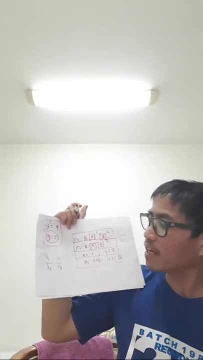 K1 over K2 is equal to R1 over R2.. Okay, Or So K1 over K2 can be simply written as K. Okay, Because these are all constant And there's no such complex in the chemical reaction. 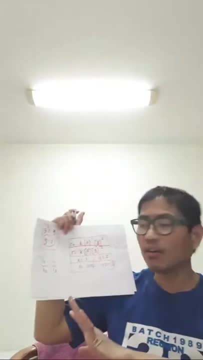 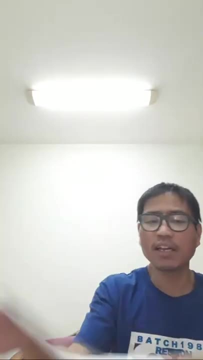 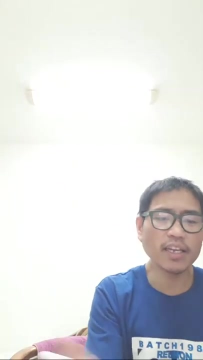 That you have another reaction. It's only one single reaction to produce a product. So K1 over K2 is just equal to K, Okay, And R1 and R2 is just equal to R- Okay. That's why in here in the general formula, 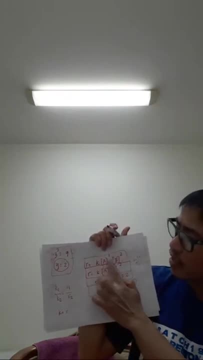 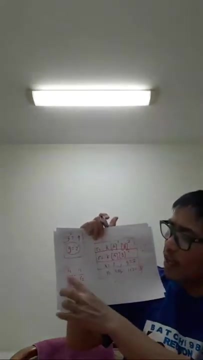 No need to put R1.. It's equal to K1. Like this, Like this Of you. If you want to make it individually, You can also get. But what I'm telling you: K1 over K2.. Constant in each reaction. 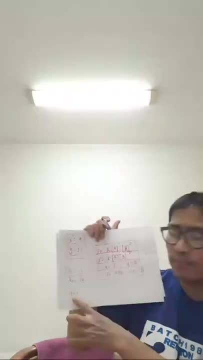 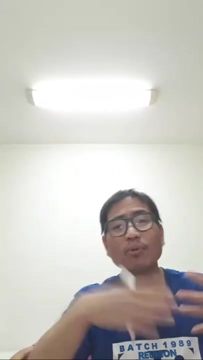 And reactant A and B. It's just equal to K Alone, And R1 over R2 is equal to R. Okay, Because you know The reactants are just single And produce other products. There's no such complications. 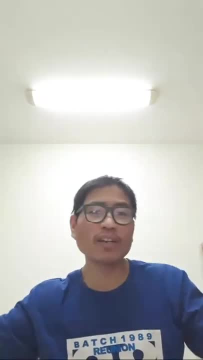 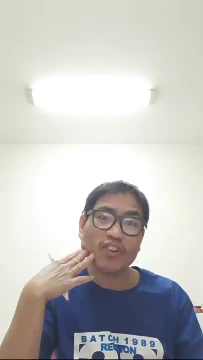 For reactants. Five reactants will produce how many products? There's no such like that. We have only two reactants. Okay, So it's going to be like that. Okay, So there's no complication in our constant. 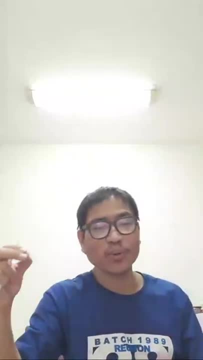 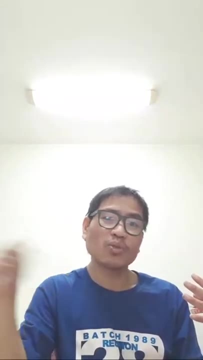 Actually we have K1, K2, R1, R2.. But, due to the proportioning, R1 over R2 is just equal to R And K1 is equal to K2.. Okay, K1 over K2 is equal to K. 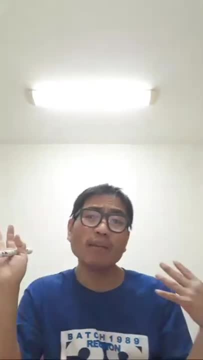 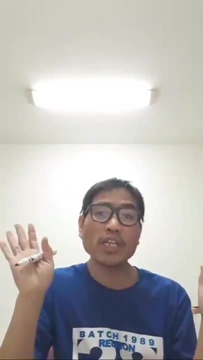 Because that's the same Ratio and proportion- Proportioning- But you cannot proportion if They don't have the same quantity, Something like that. Okay, That's the rule for ratio and proportion In mathematics. Do not do that if it doesn't have the same or similar quantities. 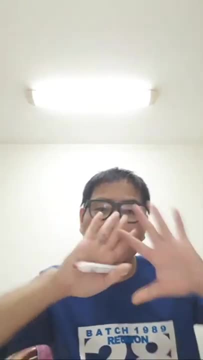 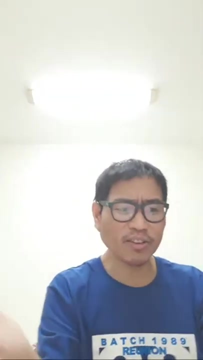 Okay, Like that. It should be basing on the similar quantities In here, similar quantities Like that, Okay. So if you want really to break down, So let's say R1.. Okay, R1 is equal to K1.. 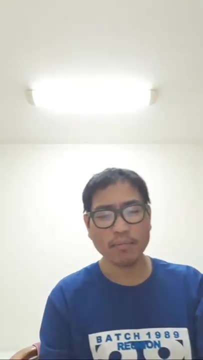 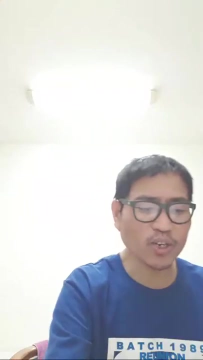 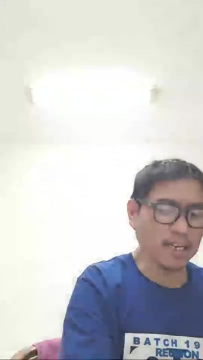 A raised to the power 1.. Okay, Equation. How many equations is this Equation 6.. Oh, equation 5.. Sorry, Equation 5.. Okay, Equation 6.. R2 is equal to K2.. B is the power 2.. 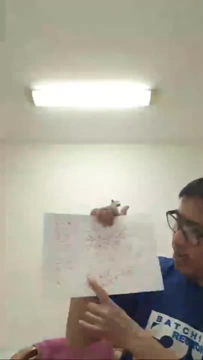 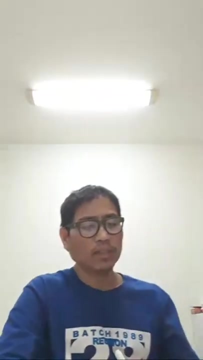 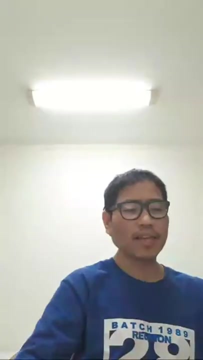 Like that, Okay, Okay, Then R1, R2.. You have also this one, And then you can combine that one To obtain the same, like this: Okay, As I told you. Okay, Like that, Or state it differently. 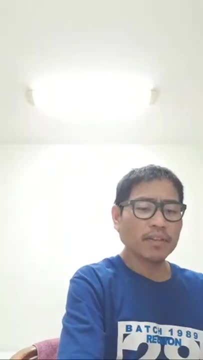 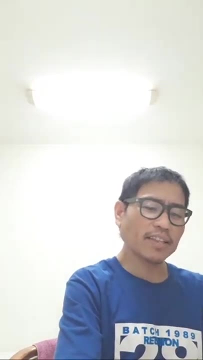 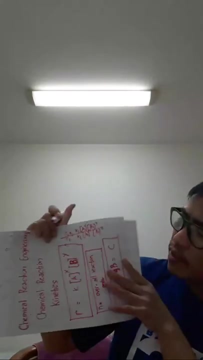 Okay, R1.. Okay, K1.. A1. B1. Charot- Okay, Then like this: 1, 2. Okay, R1.. So it's just the same. The K1, K2 is just the same. 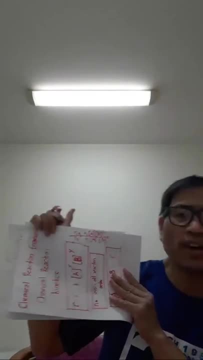 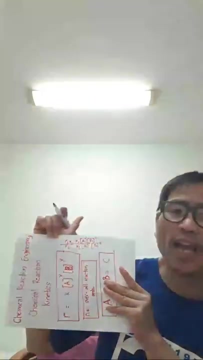 The A1, A1 in the denominator is just the same. So just put that as A alone, Right? Okay, If you put R1 over 2 as R alone, The same thing. K1, K2 is also K alone. 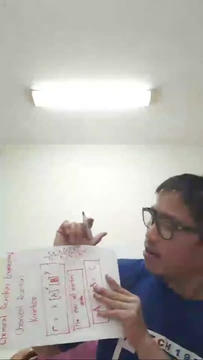 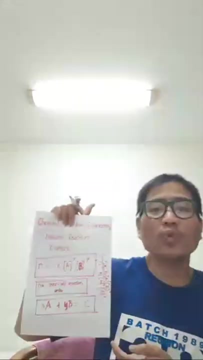 And A1 and A2 is A alone And B1, B2 is K alone. And I'm just showing you why we come up for this R, Since we know we have two equations Where the other equation goes. 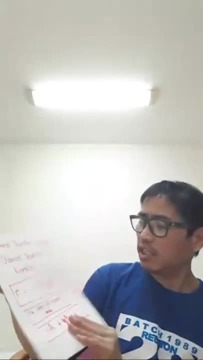 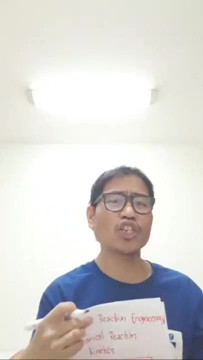 Something like that. Just because of this ratio and proportion, This one, Okay, Like that. Now we go now to the relationship. This is also important because some of the problems also and questions will be like this also: Now, if you increase the ratio, 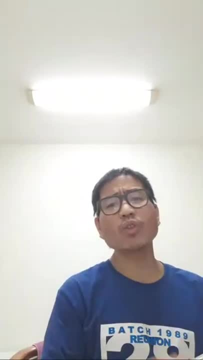 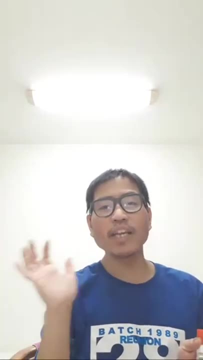 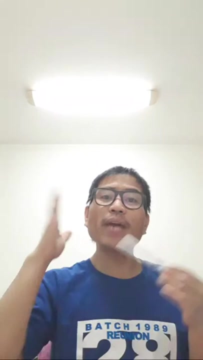 If you increase the rate constant of the equation K, what will happen for your chemical reaction? Okay, Your chemical reaction will become faster. Okay, If there is a small value of K, which is your rate of equation constant, your reaction will be faster or higher. 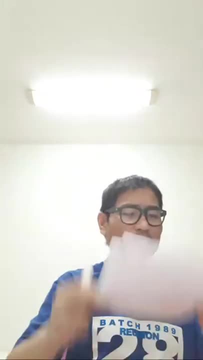 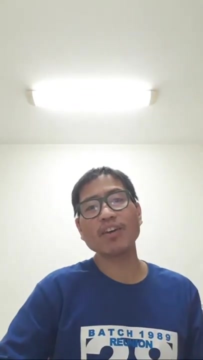 So we can say that automatically that, okay, K is inversely proportional to your rate of reaction. So we can say that automatically that okay, K is inversely proportional to your rate of chemical reaction. Okay, Or rate of low chemical reaction. 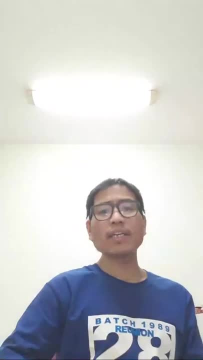 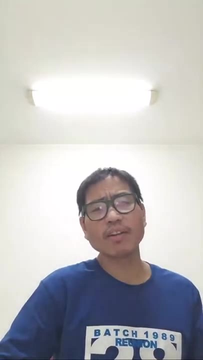 For example, if the problem gives you a very small K, it is expected that you have a higher rate of low chemical reaction, Or rate of chemical reaction, Or faster chemical reaction. It's going to be like that. Don't be confused with the terms. 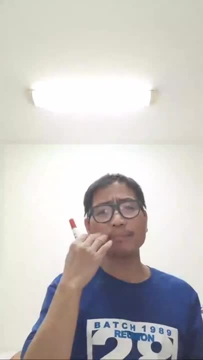 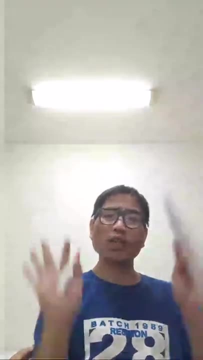 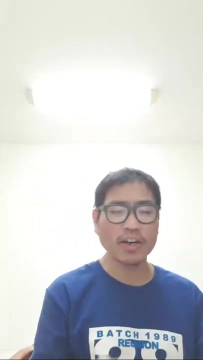 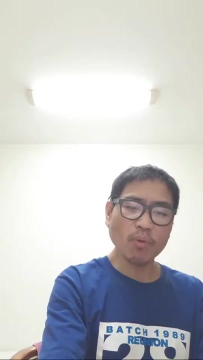 Okay, Again, if you have a high constant, your rate of reaction Will become slower or lesser Because inversely proportional with each other, Not directly proportional with each other. So the relationship is inversely proportional with each other. K is 1 over rate of the reaction. small letter R. 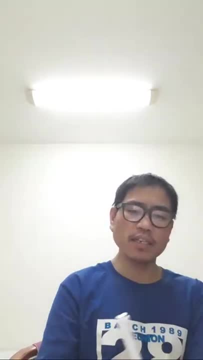 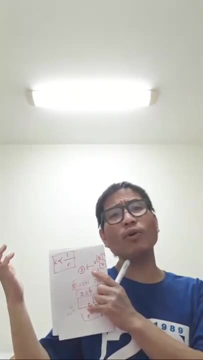 This one. Bear this in mind, Okay, Because somewhere along your computation you get the final answer. Then it's not also logical, Oh my God, Why this is higher, Based on my theory, it's become big, So you have wrong solution. 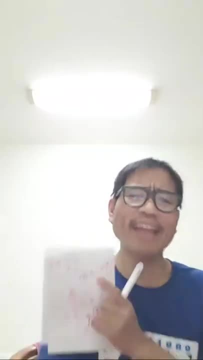 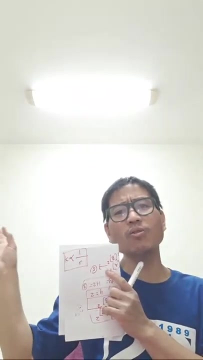 Okay, So you need to review again. Sometimes it's not enough to get the answer. You have to think also: Oh my gosh, Why it's become low and my initial reaction is like this- And why it's still lower. 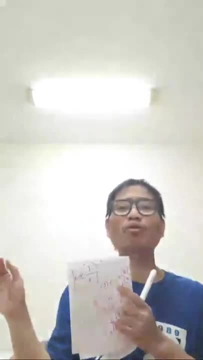 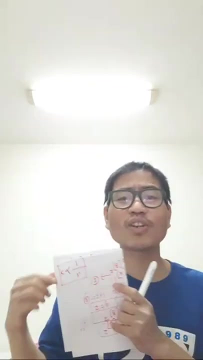 And I have a very high K. Like that It's not enough to solve that. You know everything, The formula, Then you go: like that There's something wrong with your theory. It doesn't match to your final answer. The theory is governed. 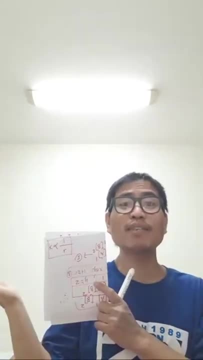 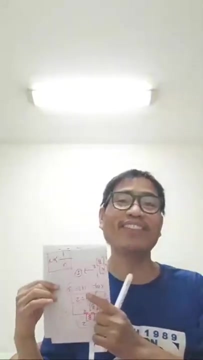 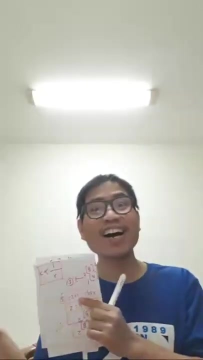 On that particular topic. I think that's most usual mistakes of some examiners, including me. Okay, Especially when we get in hurry. Okay, Like that We don't examine anymore that it's going to be logical, reliable or valid to get that answer. 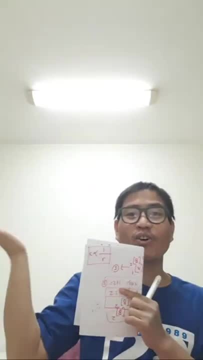 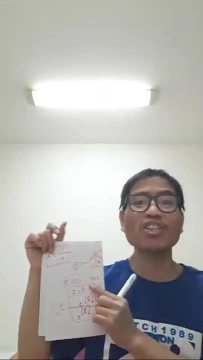 Even though our solution is, we feel it's correct because we're using the correct formula, But it is not really that enough. You have to, you know, evaluate. You have to evaluate the relationships, All chemistry problems like that, huh. 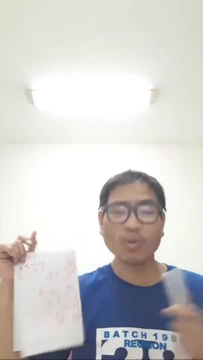 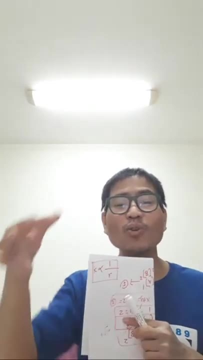 Even the higher chemistry, or even unit operations, Something like that. also Bear that in mind. The relationship could either be directly proportional or inversely proportional, So that you can determine your answers: High, low, big, small Like that, And it should be valid. 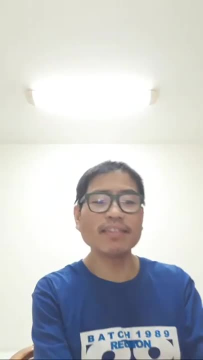 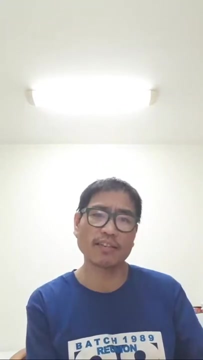 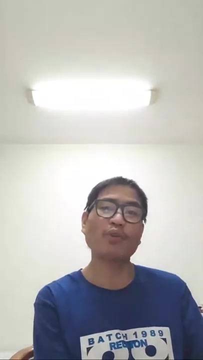 Okay, Something like that. So this is enough for the overview, or the basic foundation, of chemistry, Chemical reaction engineering or chemical reaction kinetics. Okay, In my next live streaming I will be able to give specific examples of the chemical reaction And we apply this basic interpretation of this chemical reaction engineering. 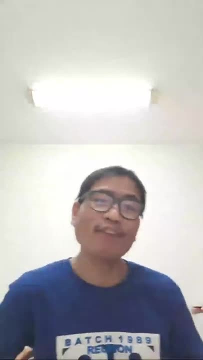 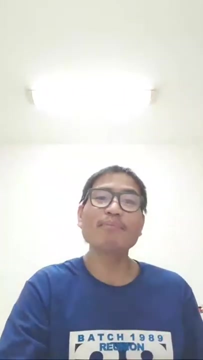 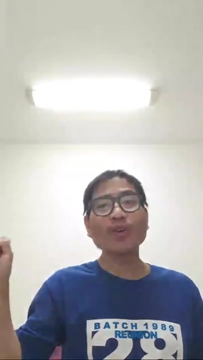 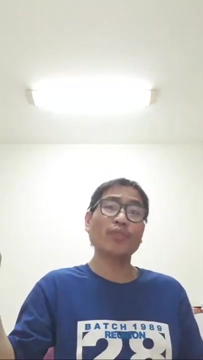 And then bingo, we can solve simpler to average problems for this chemical reaction engineering problem. I cannot assure you difficult problems, because me also. I find difficult this topic and subject And I was in my college days. Okay, Like that, I am assuring you, you will learn a simpler to average type of chemical reaction engineering problems already. 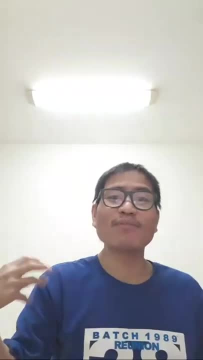 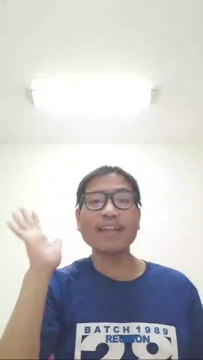 Okay, The difficult one, never mind. Okay, As long as we have the, you know, the basic foundations, As I told you early or earlier a while ago. okay, the examination- you know bodies- will not give a lot of difficult problems because all will fail. 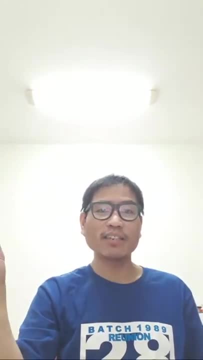 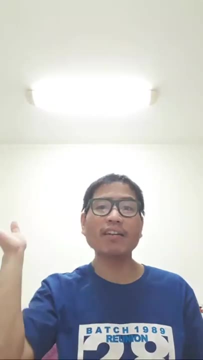 Okay, That's why it's called regression, Regulating or regulated commission, Something like that. It's impossible. They will give different all difficult. No, it's not, It's our own mind only that tells us, oh, it's difficult. 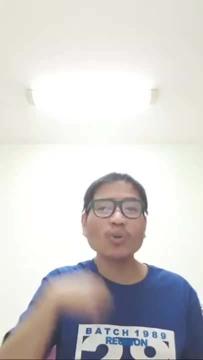 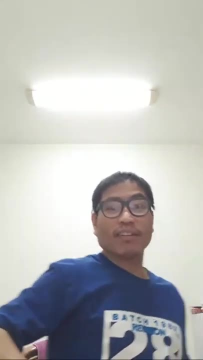 Oh my God, It's the psychological effect, But actually it's more on simpler to average, Only small or difficult questions, Okay, Like that. Okay, Only regulated, but not all difficult. Okay, If that is the case, nobody will pass. 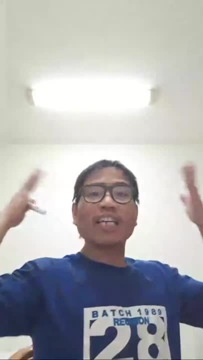 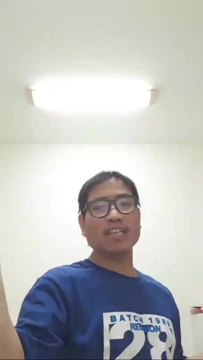 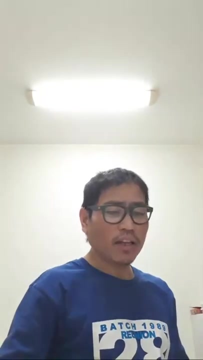 Okay. If all are difficult, Just try that too, Inculcate in your mind: Okay, All types of examination, not only, are limited to PRZ, Board Engineering Examination- Okay. Or Engineering Licensure Examination: Okay. Thank you so much for listening.